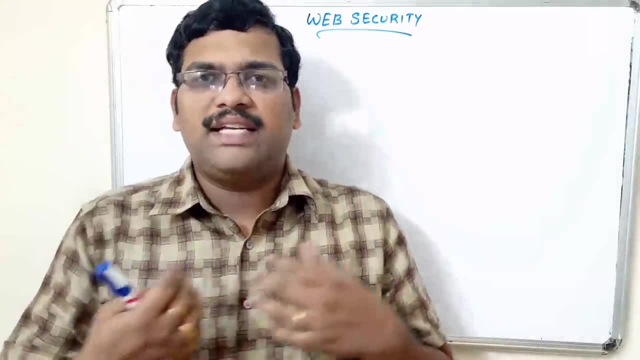 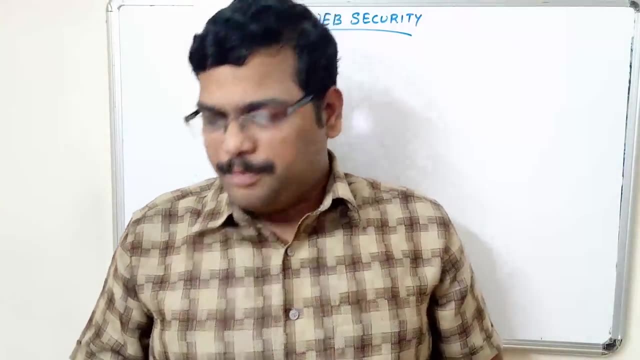 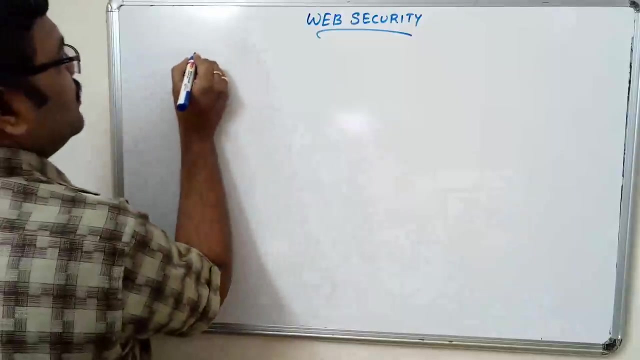 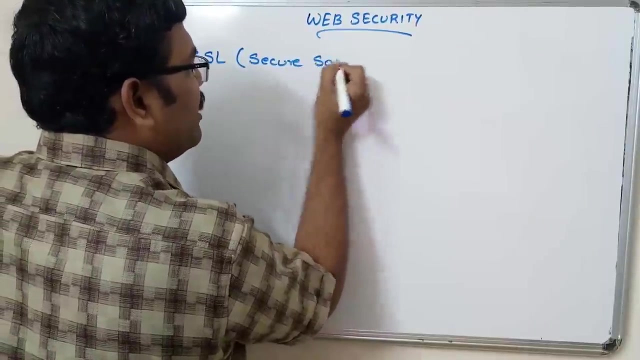 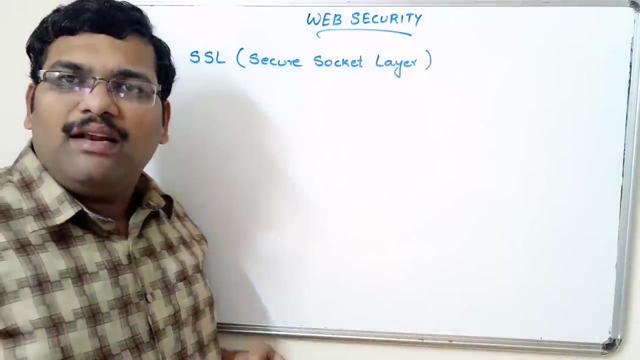 client and server example. so the, as usual, the client will send the request to the server and the server will provide the service to the client. So for this purpose, we will use a one protocol that is called SSL protocol. SSL that means secure socket layer. So by implementing this SSL, we can. 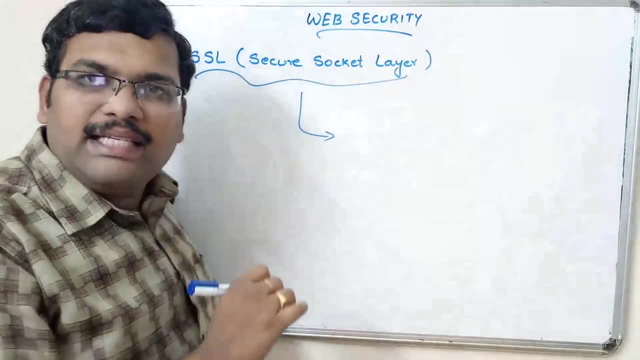 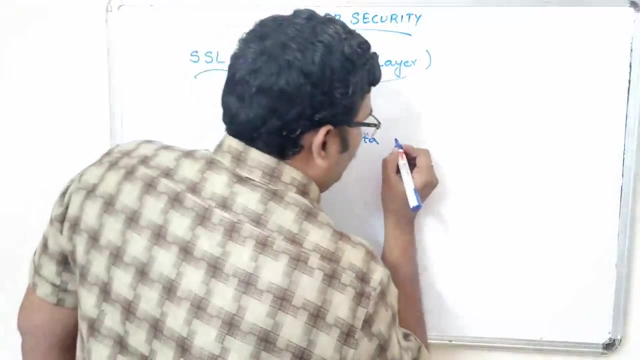 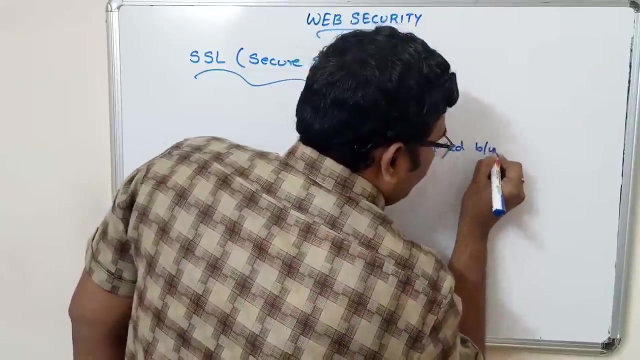 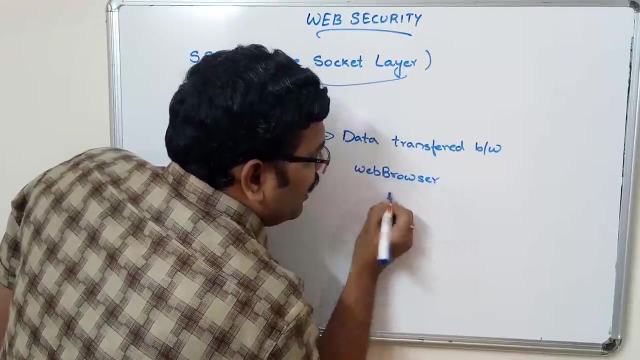 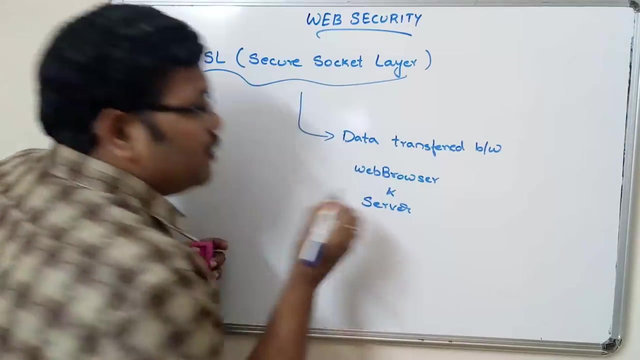 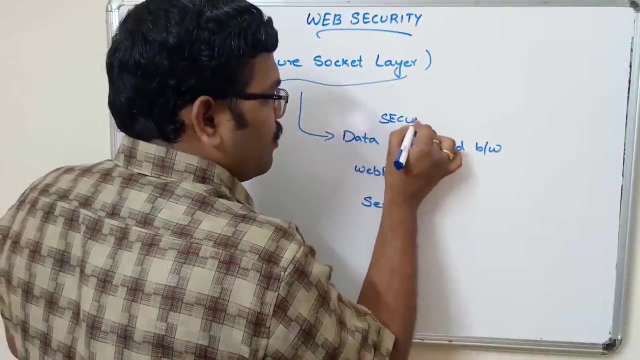 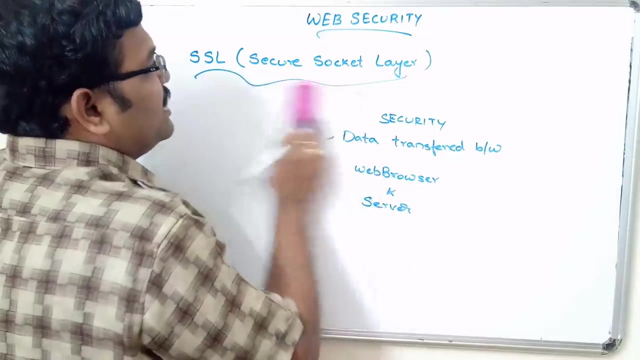 also this secure socket layer will act as I mean will provide the security for the data which is transferred between the web browser and server. So by implementing this secure socket layer, we can provide the security for the data which is transferred between web browser and the server. So this SSL is implemented by using a different 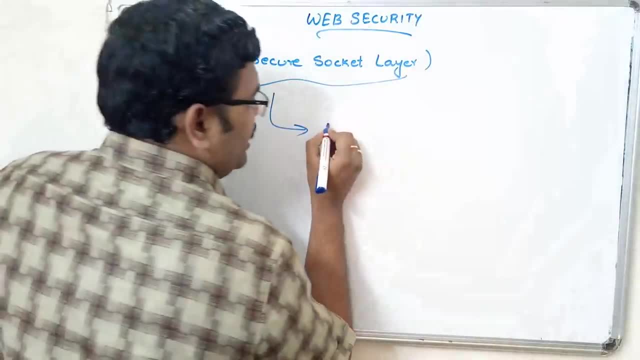 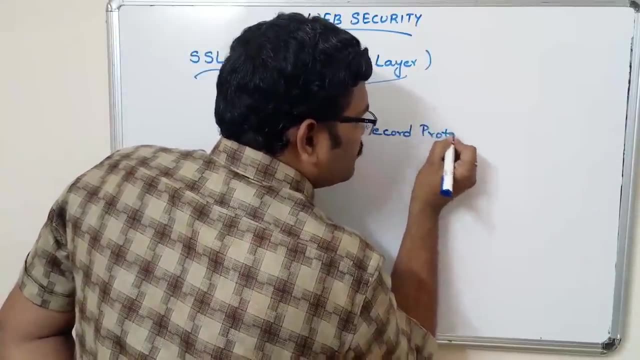 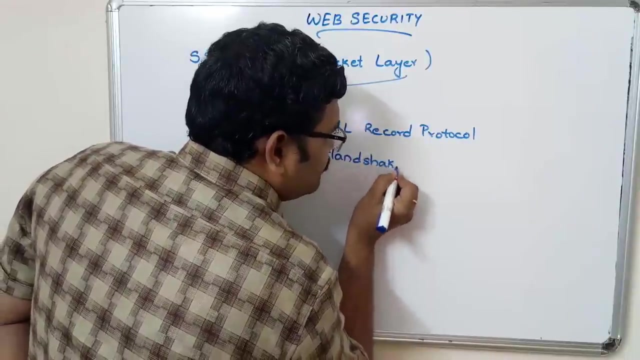 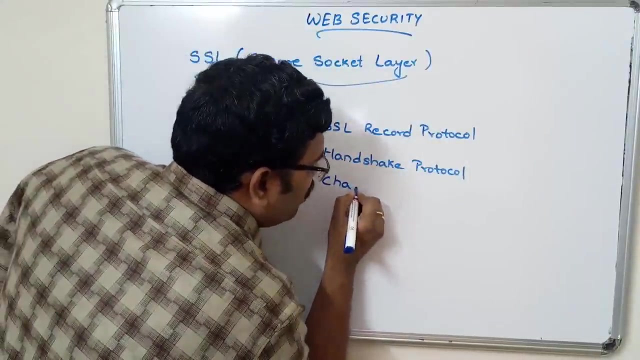 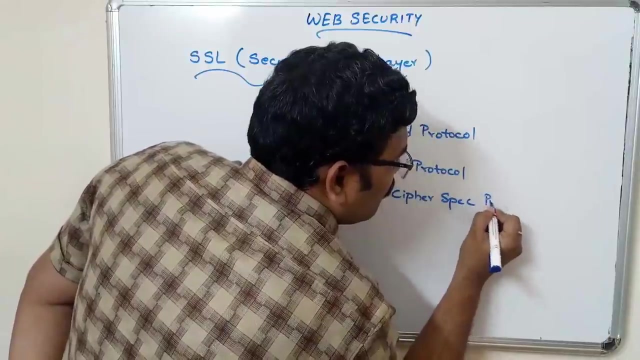 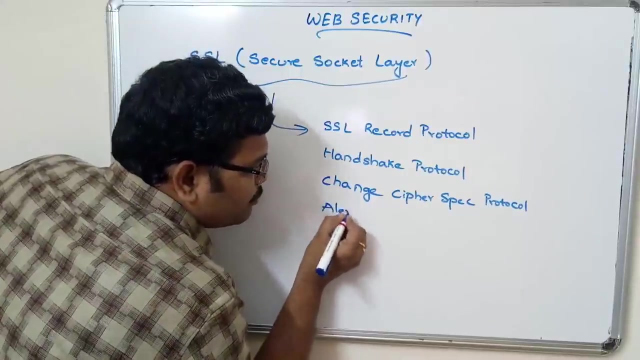 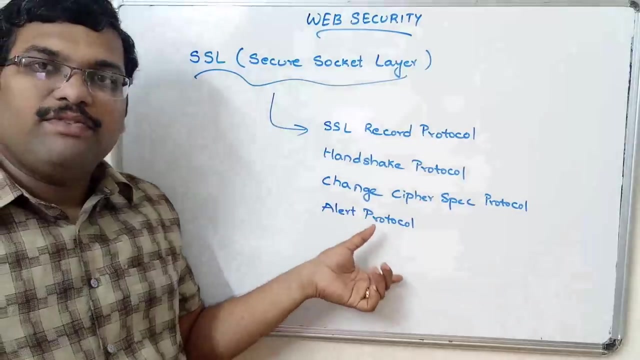 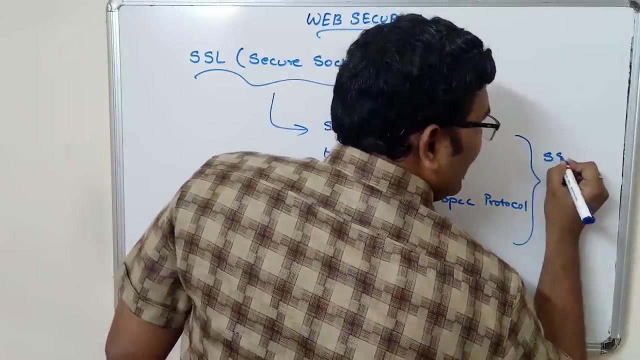 protocol. So it includes a different protocols. One is SSL record protocol and another one is SSL record protocol, Handshake protocol, Change cypher spec protocol And next the alert protocol. So all these protocols will be included in this SSL secure socket layer. So this we call it as SSL protocol stack. 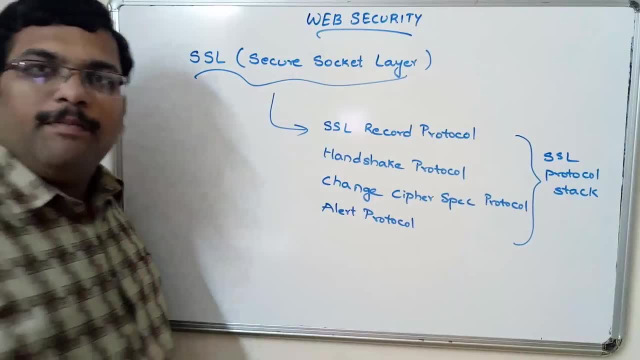 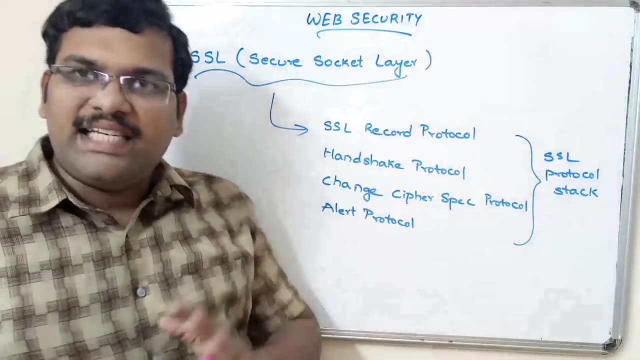 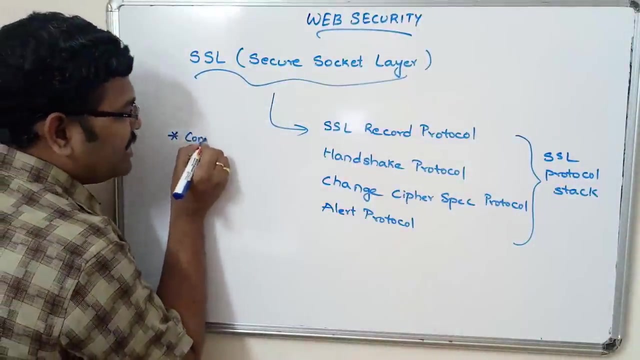 So this will be implemented just above the TCP IP and just below the HTTP. So before going to this SSL, the two main concepts must be implemented: SSL protocol stack, That is first. one is connection. So these are very, very, very important while implementing this SSL. 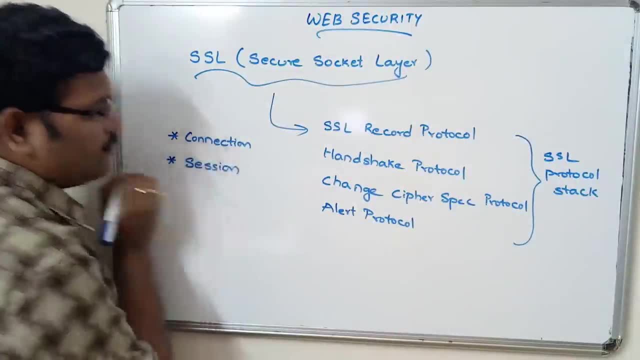 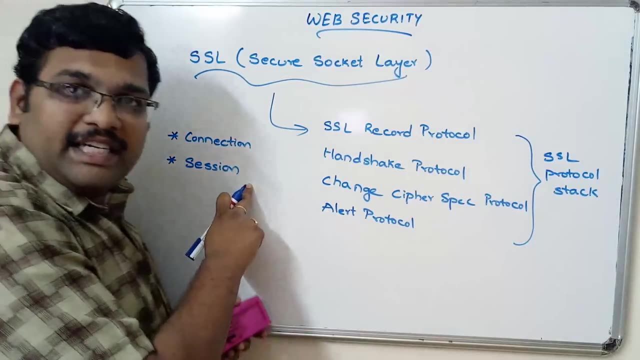 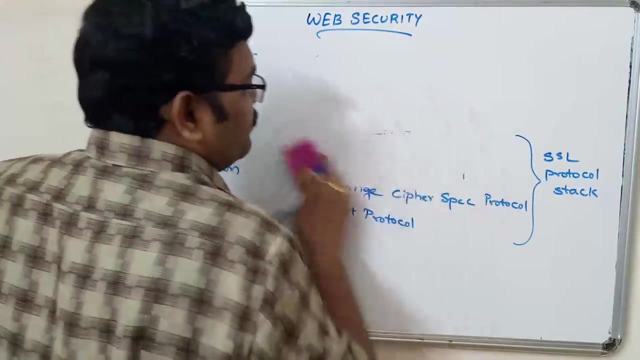 And session. So what is a connection and what is a session? So first we will look at this connection and session and then we will move on to the different protocols. So, as we know, In order to commit this protocol To communicate both the client and server, 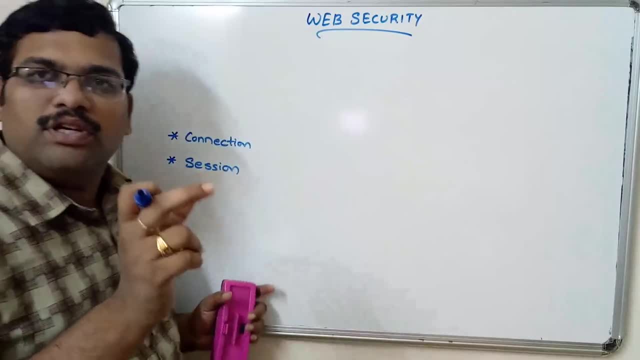 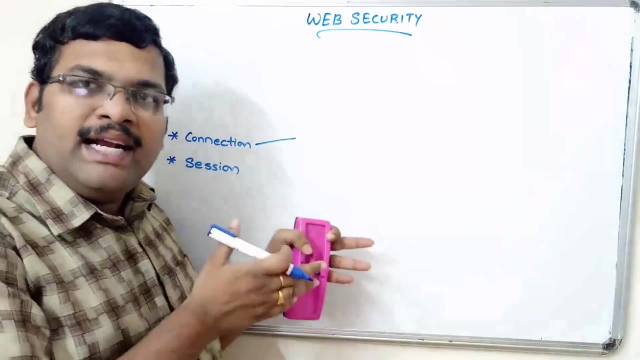 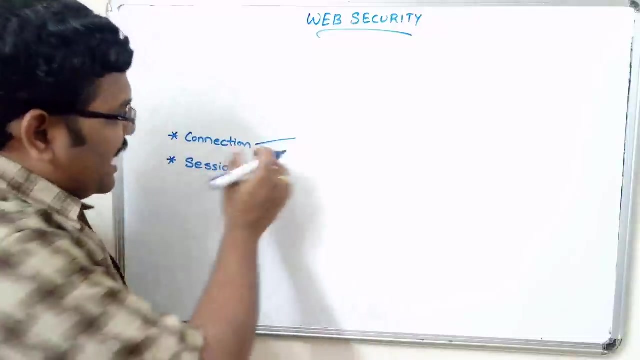 The first thing is the transport to provide the service That we call it as connection. So first the connection should be established between the client and server So that the client can communicate with the server and the server can communicate with the client. So this connection is a transport. 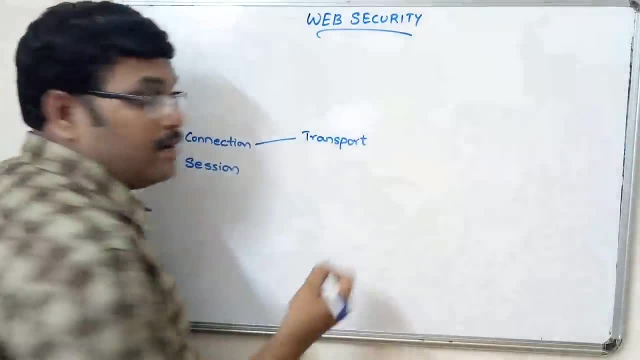 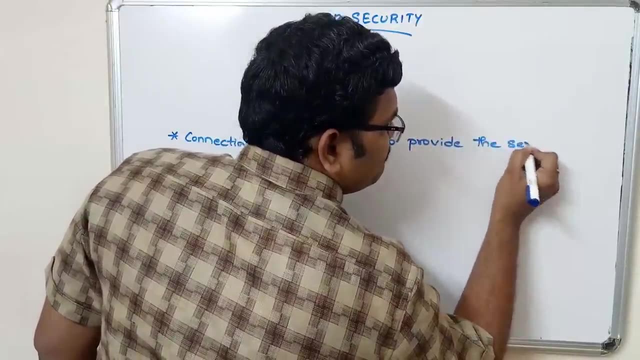 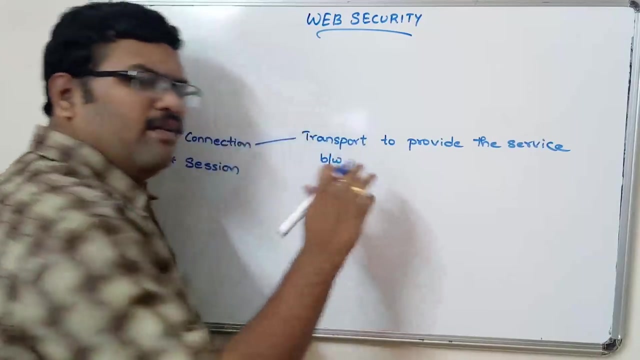 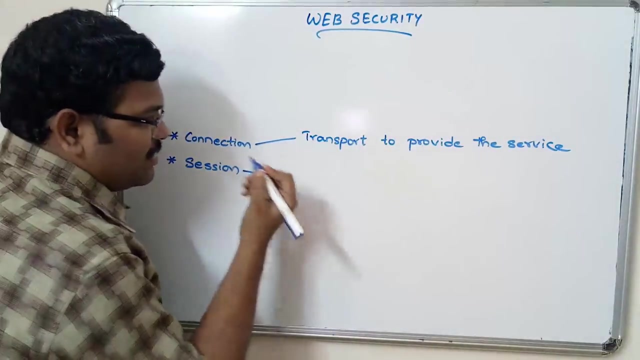 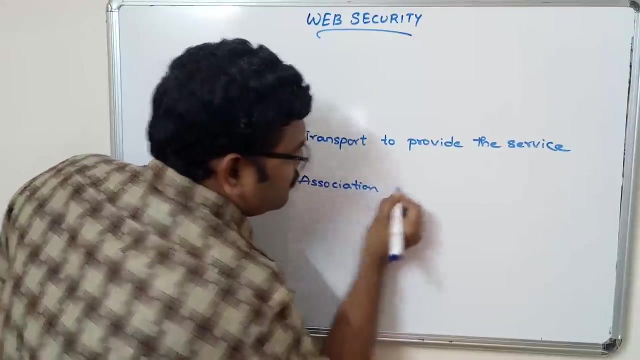 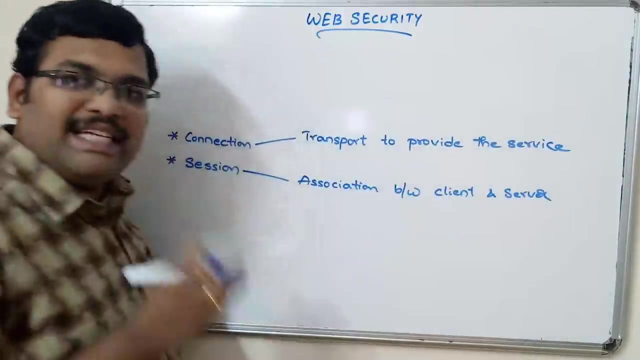 To provide The service Between the client and server, Between We can say client and server, or between two clients, whatever it may be. So session, A session, is An association Between The client and server, So one session will be created. 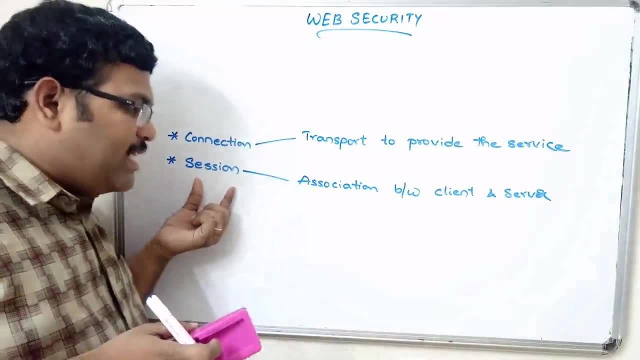 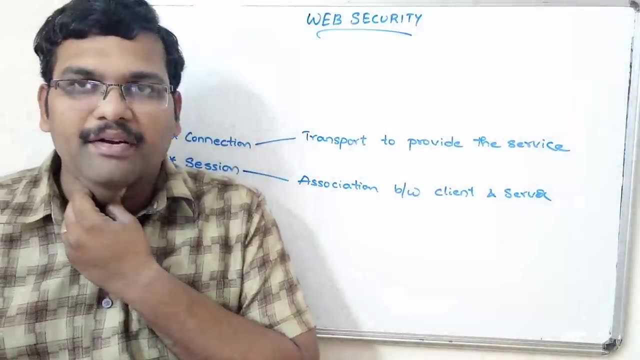 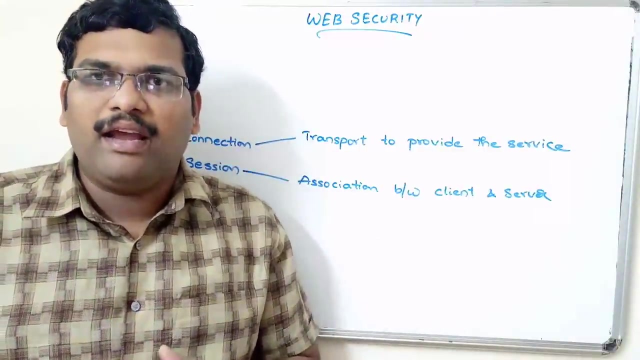 And, Based upon this session, The client and server will be communicated. So, generally, this session, we call it as a temporary time period, Right? So If you observe the bank sites, So if you log into your net banking and just Keep the 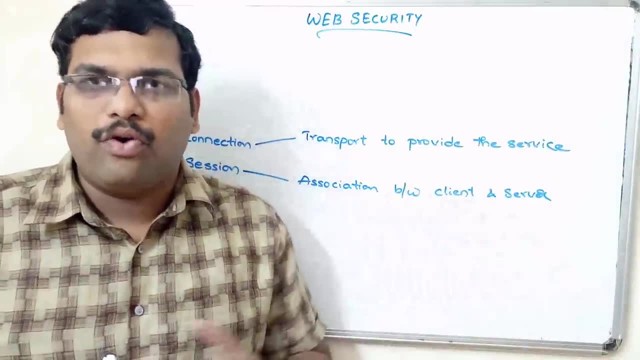 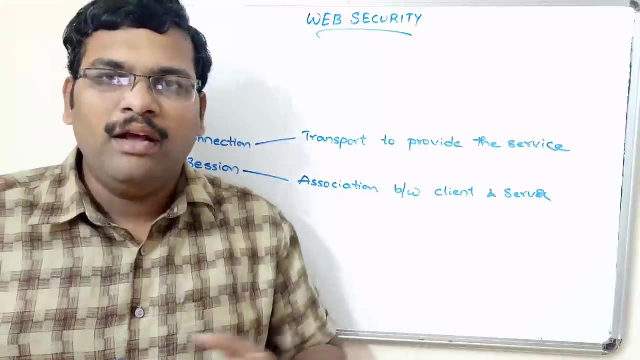 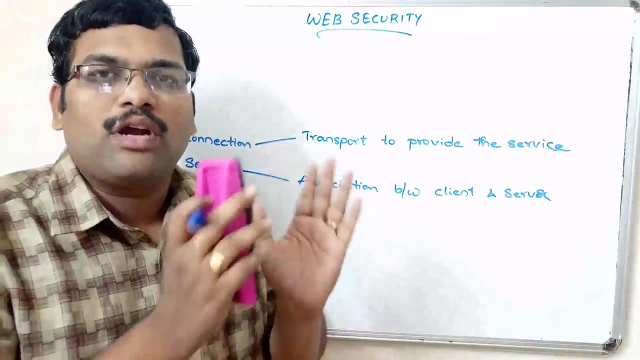 Net banking site idle for Three to four minutes. Automatically you will get the message, alert message- that Your session has been expired, So re-login To use the service. So here the session means Up to some time. The client and server should communicate each other. 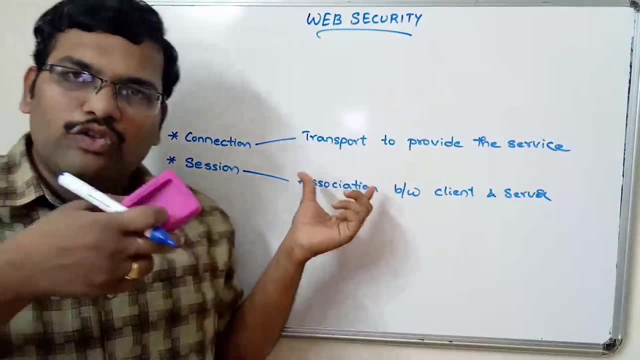 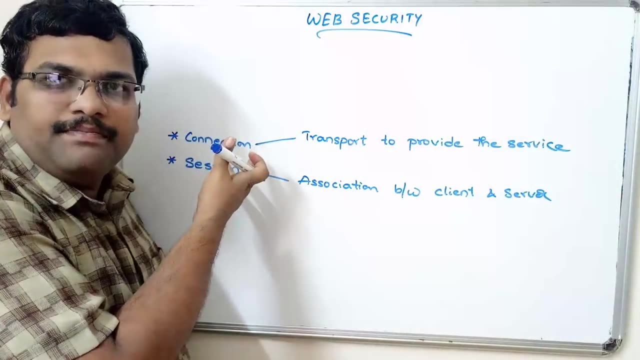 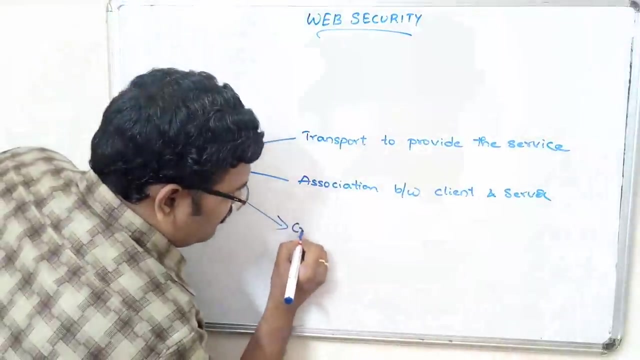 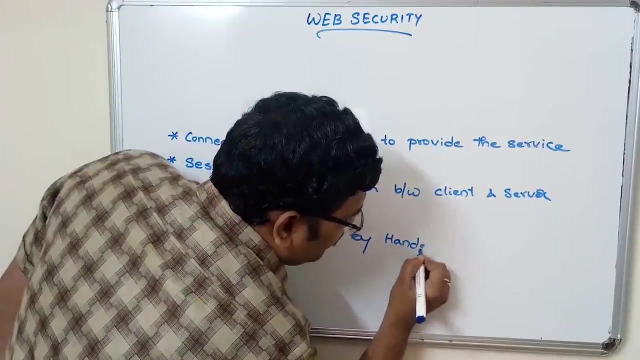 Right So that we call it as an association Between the client and server. So this session consists of A number of connections, The multiple connections Right. So These sessions will be created Or generated By handshake protocol. All the sessions will be. 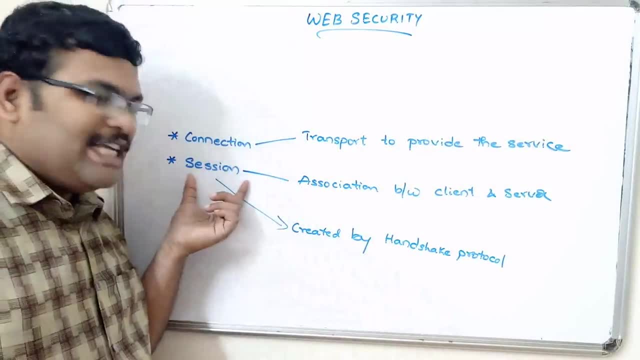 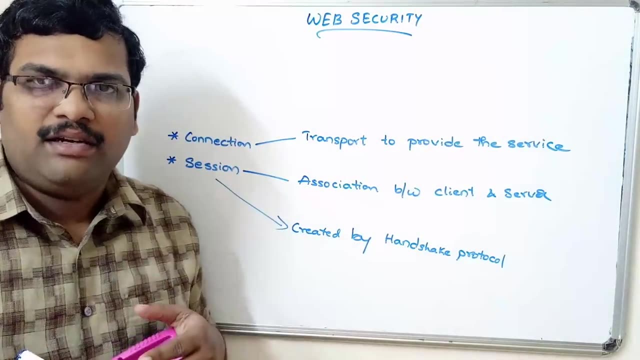 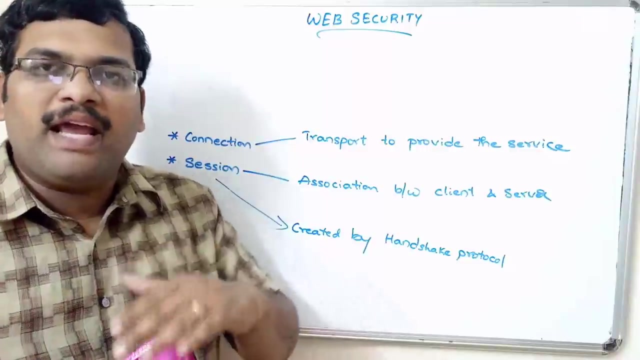 Generated by handshake protocol. So once a session has been created, Automatically It consists of multiple connections, A number of connections. So Every session will be identified By using some parameters Which can be used by All the connections In that particular session. 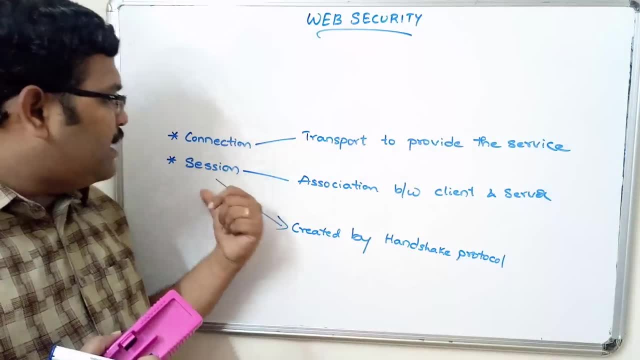 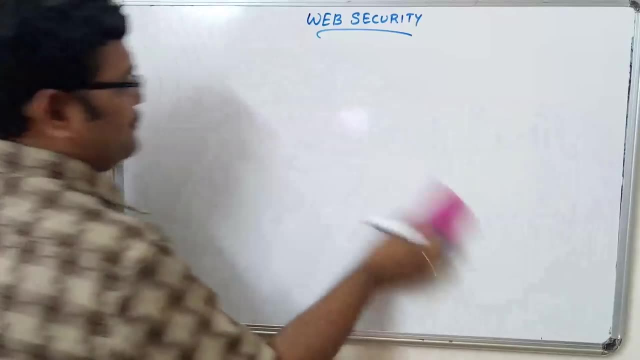 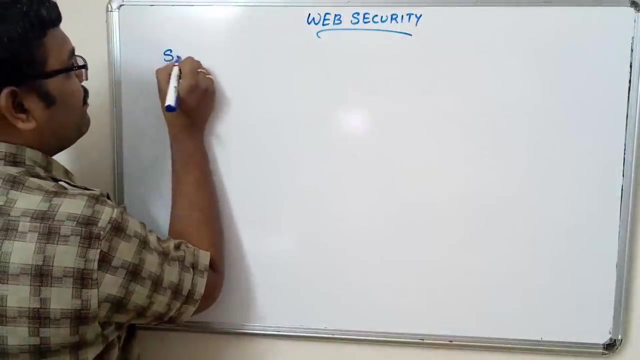 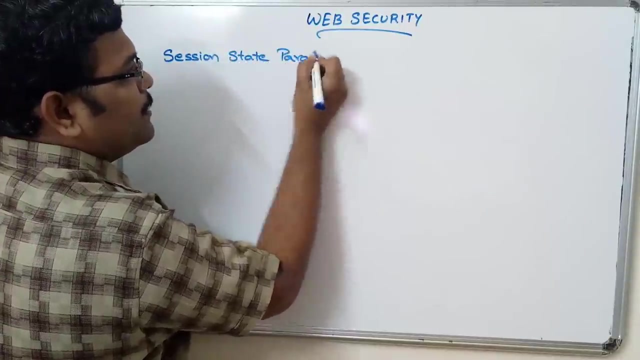 So let us have a look on Parameters of session And the parameters of connection. First, Session state parameters. So what are the parameters Associated To identify the session Right? Session state parameters. Session state parameters Right. The first one is: 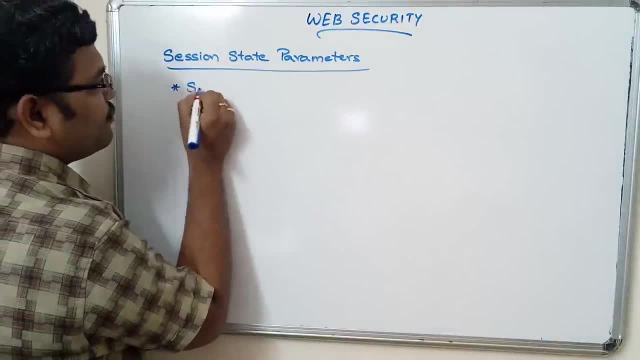 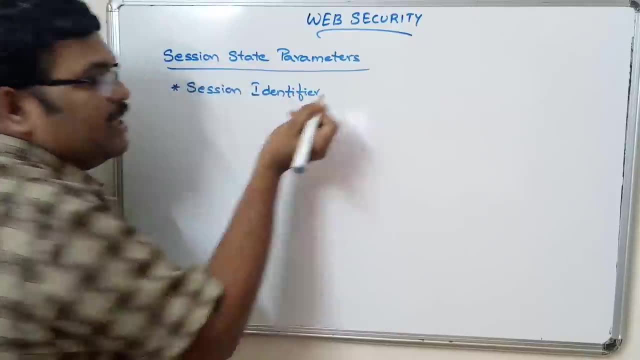 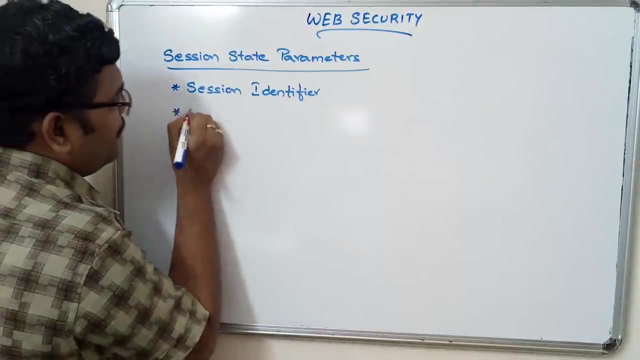 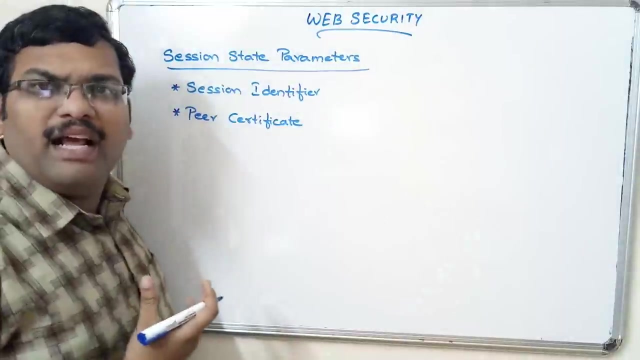 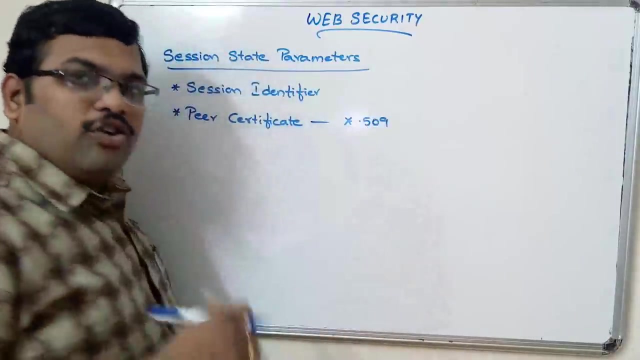 Session identifier. It is a byte sequence To identify that particular session. Next Page certificate, Page certificate, Page certificate: Here Page is nothing but a client, So client certificate So, which is generally X.509 certificate, So in this certificate. 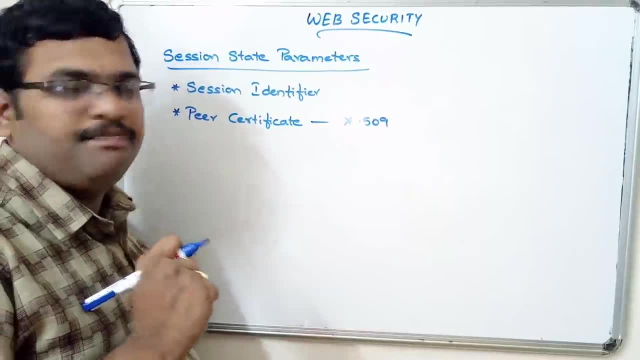 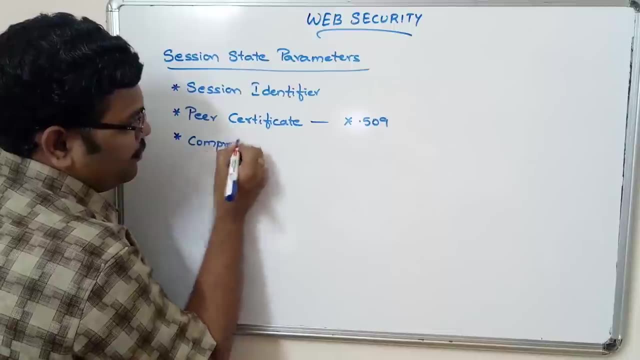 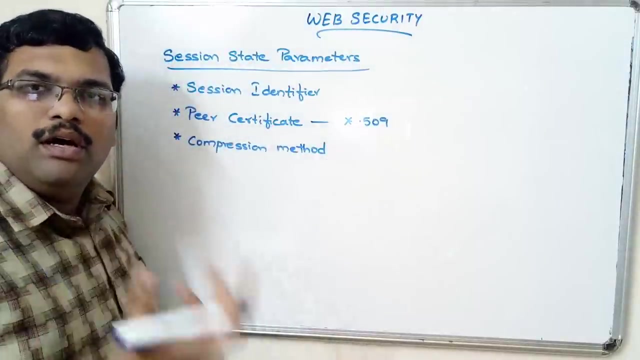 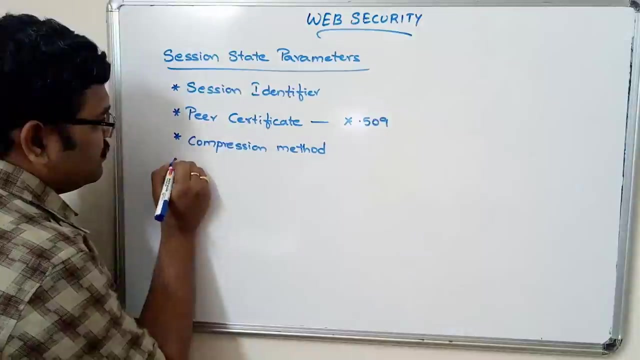 We have The public key of the client As well as the signature algorithm parameters. The next one, Compression method. So this parameter Is used to Say the compression algorithm used Before the encryption In the SSL. So this Compression is an optional thing. 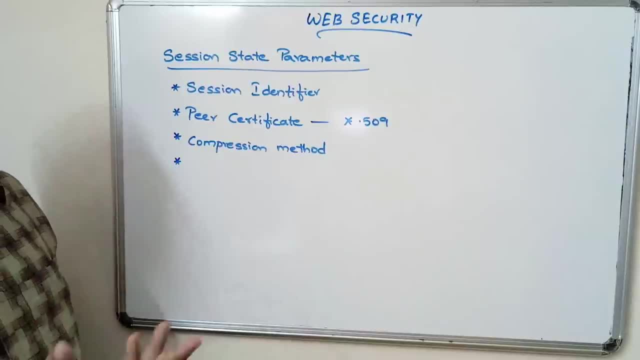 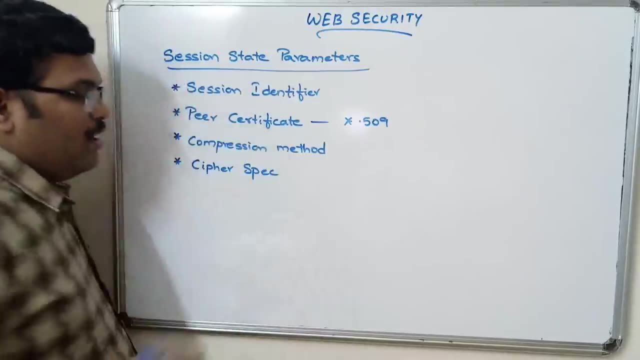 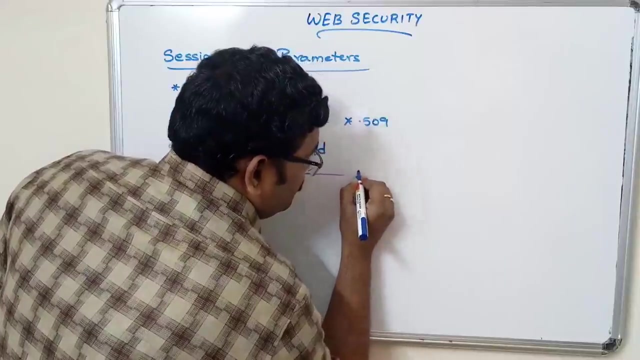 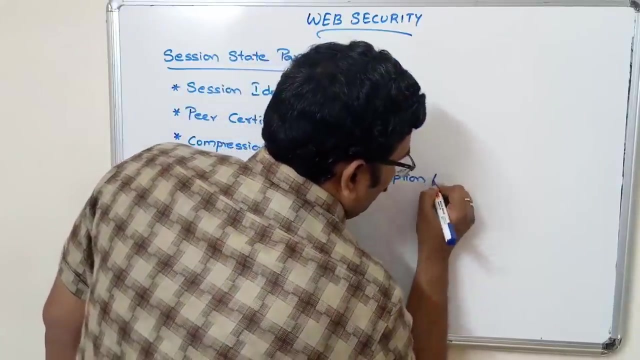 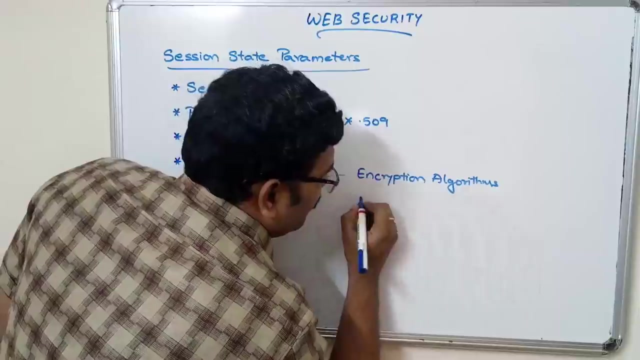 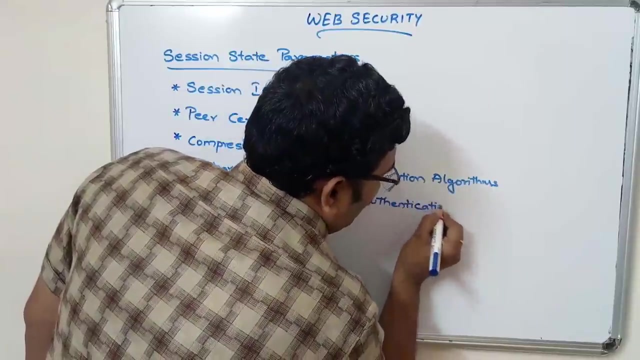 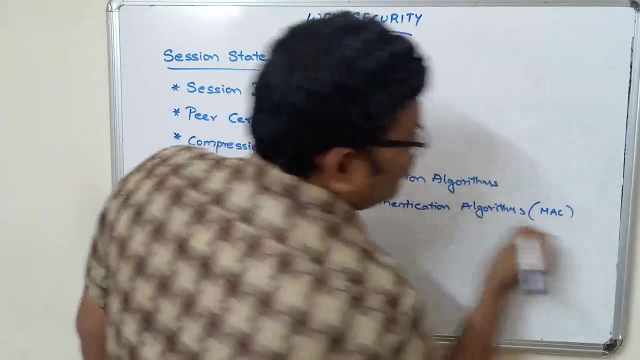 So it can be Applied, or it can, It may not be applied. Next, Cipher spec. Spec means Specification, So here we can have The Encryption algorithms And Authentication algorithms, So this can be The MAC algorithms. 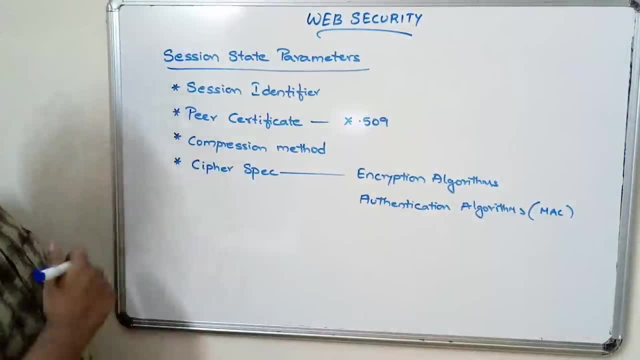 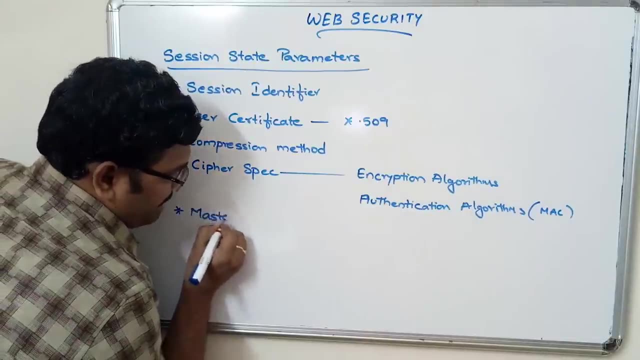 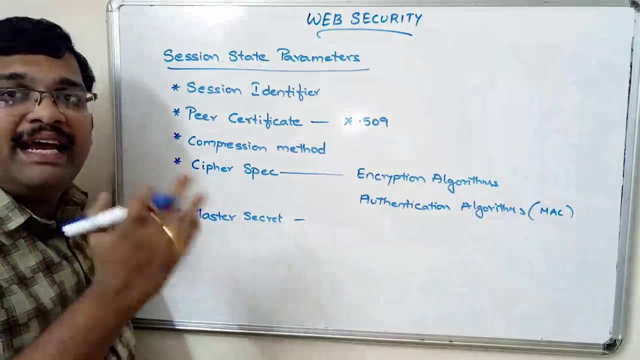 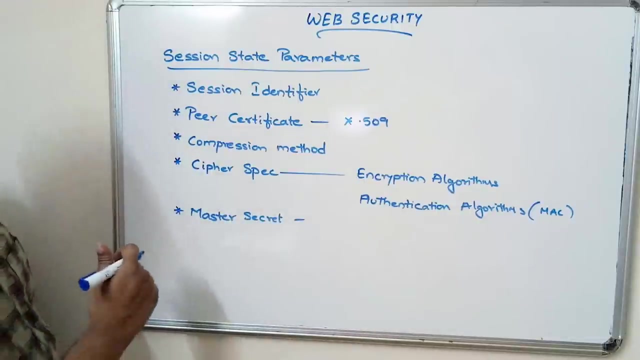 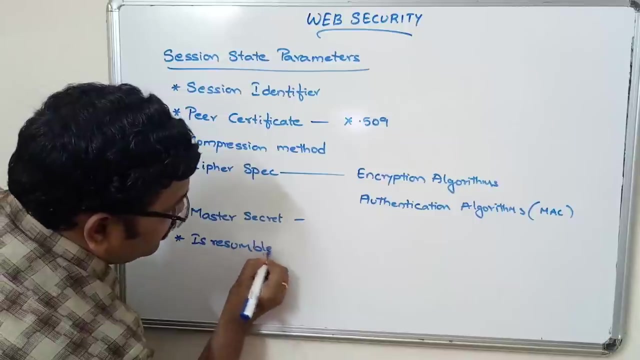 Or hash algorithms Right Next Cipher spec and then Master secret. So which is the secret key Shared between the client And server? So this is the secret key which is shared among The client and server Is Resembled. 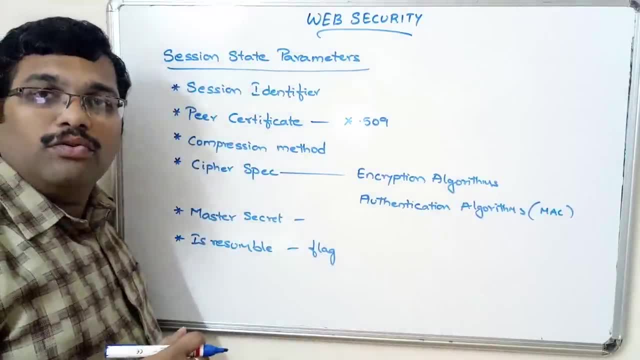 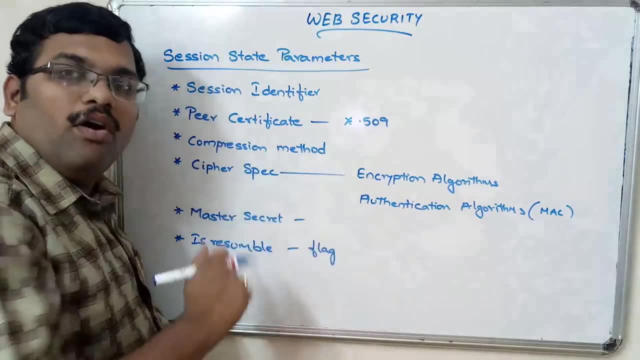 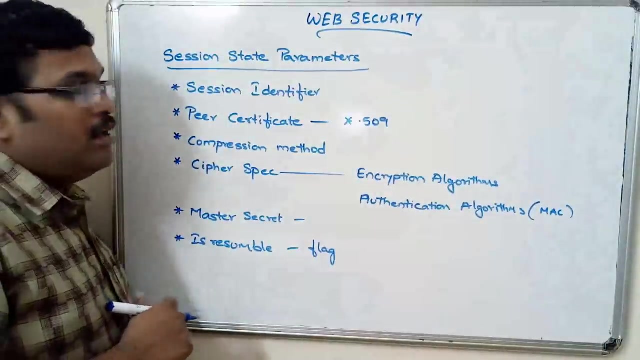 So this is a flag Which is used to Know whether the new connections Can be, or new sessions can be, Established by this particular session Or not. So all these are the different Session state Parameters Now. so these parameters. 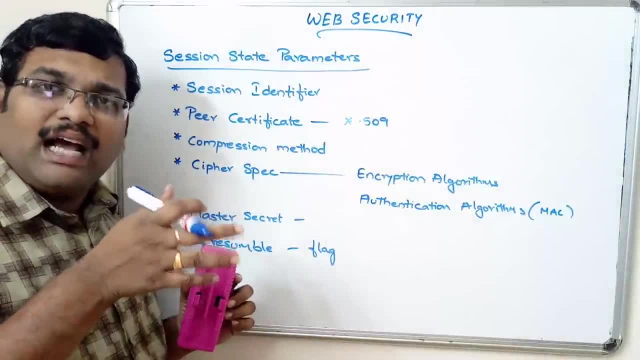 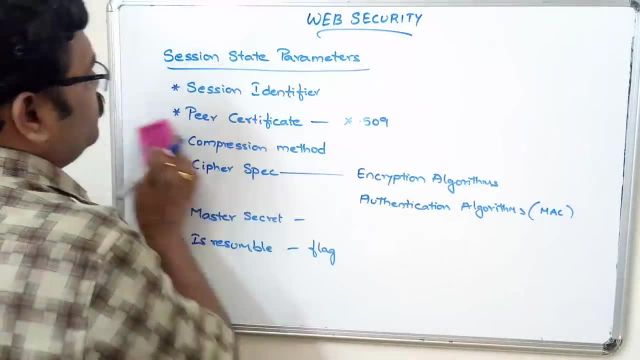 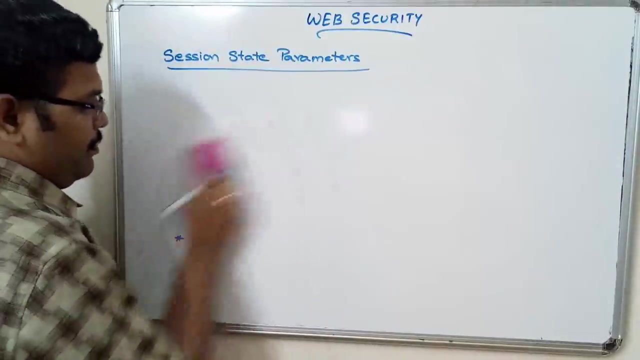 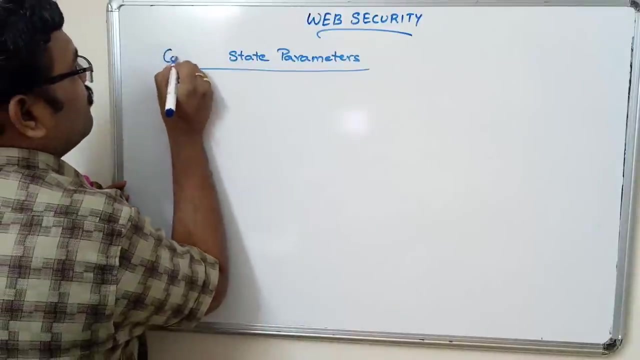 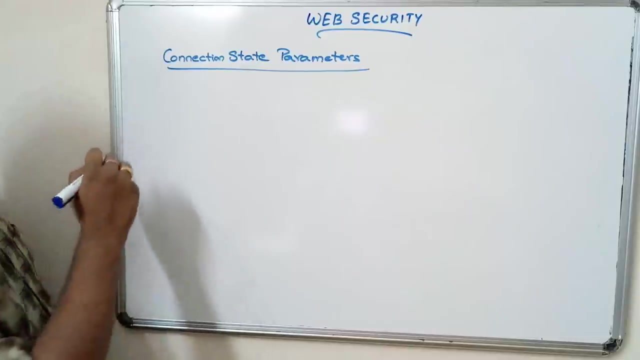 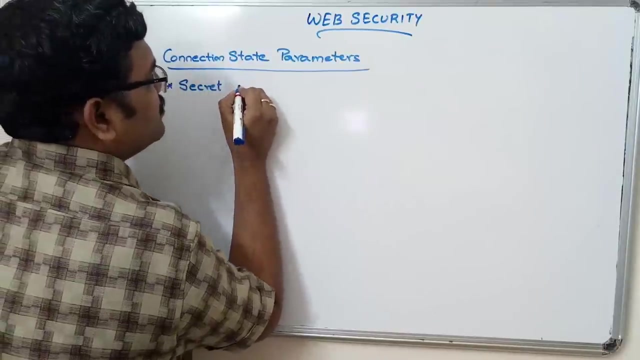 Are commonly shared by each And every connection Associated with this particular Session. Now let us see the connection state parameters. So what are the connection state Parameters? Connection state Parameters. First, one Secret, Secret, Secret, Secret. 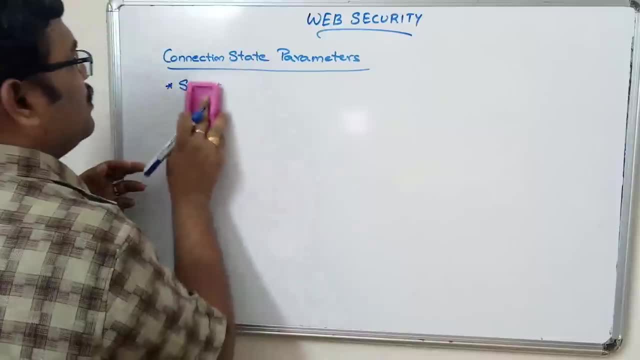 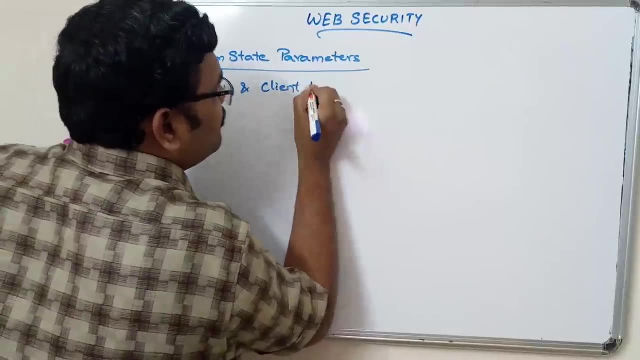 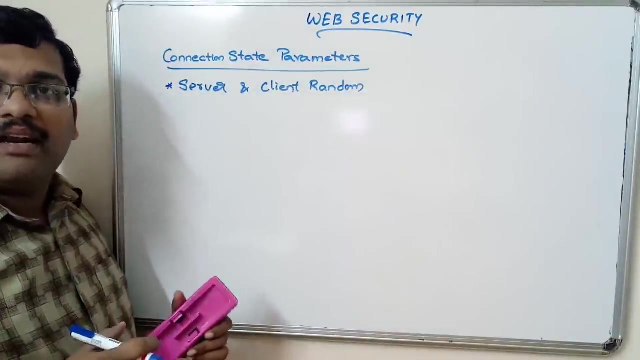 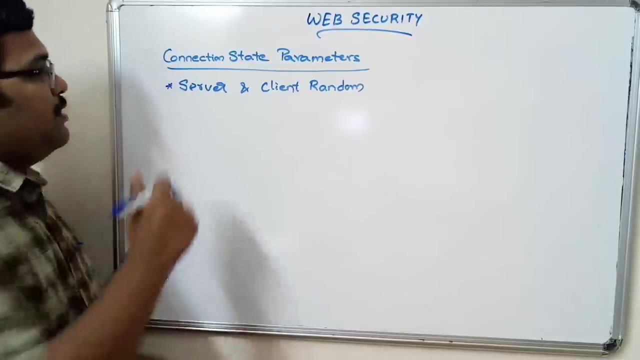 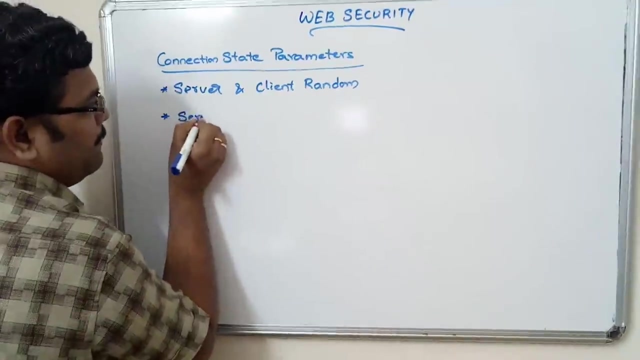 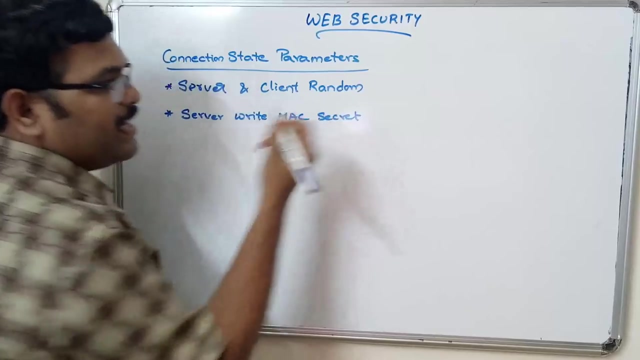 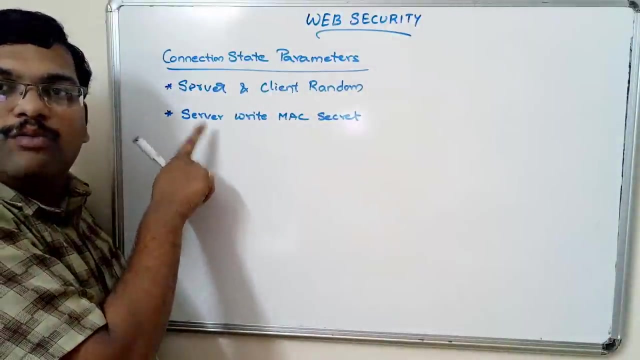 Secret Secret Secret Server and Client random, Client random Server And client random Byte sequences which are Associated with the particular Connection Or associated with the. The next, the server and the client random Server write MAC secret. So this is the MAC which is generated by the server for the data which is sent by the server. 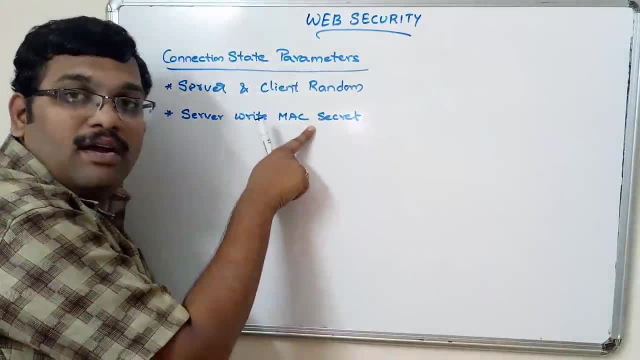 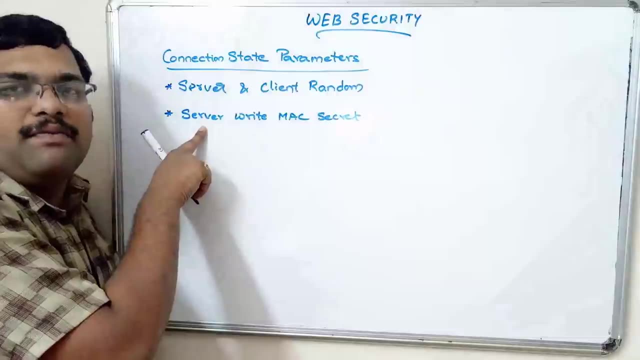 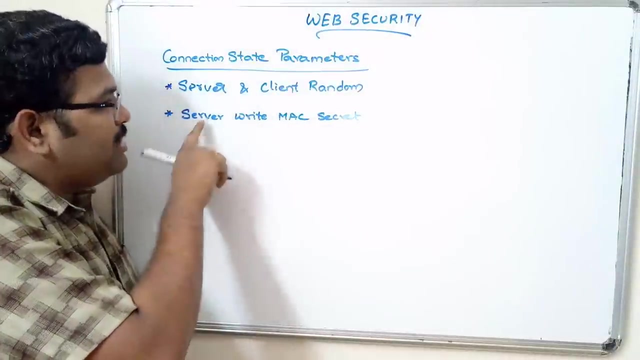 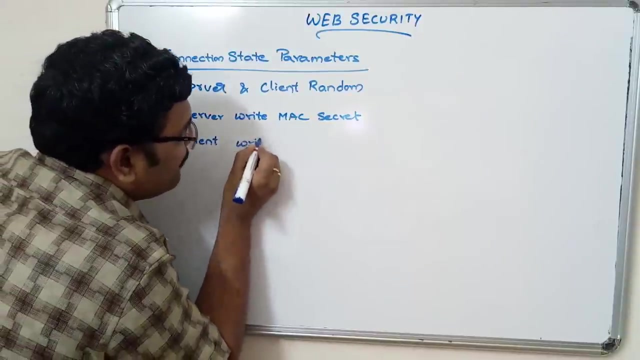 Okay, So don't get confused. This is the MAC which is generated for the data which is sent by the server. So here the sender is the server, So sender will generate the MAC. So this MAC is generated by the server. Similarly, client write MAC secret. 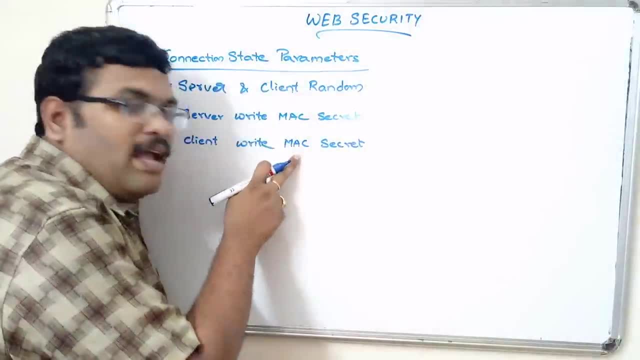 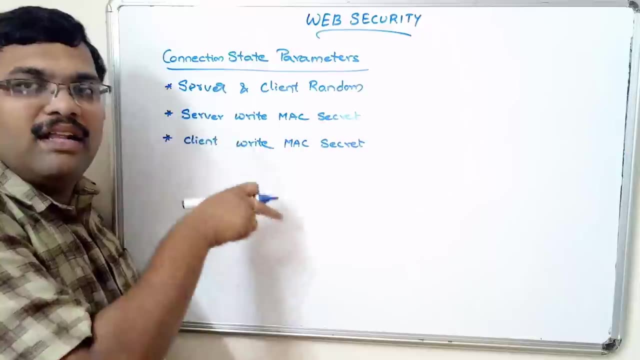 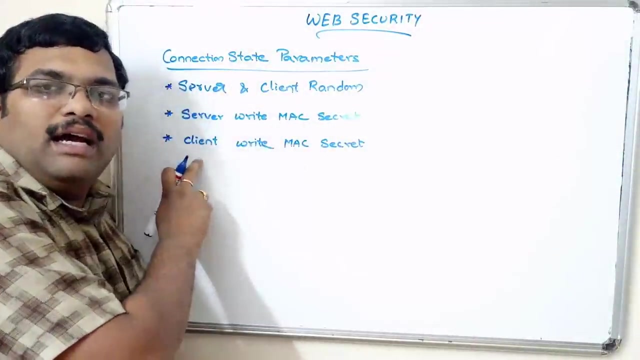 So here the client. MAC write secret means this is the MAC generated by the client for the data which is sent by the client. So here the sender is the client, So MAC which is generated for the data at the client side Right Next. 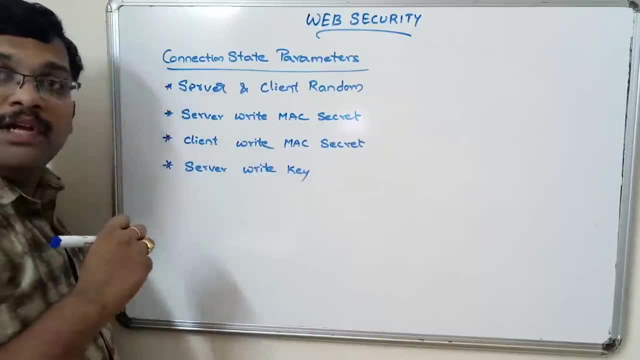 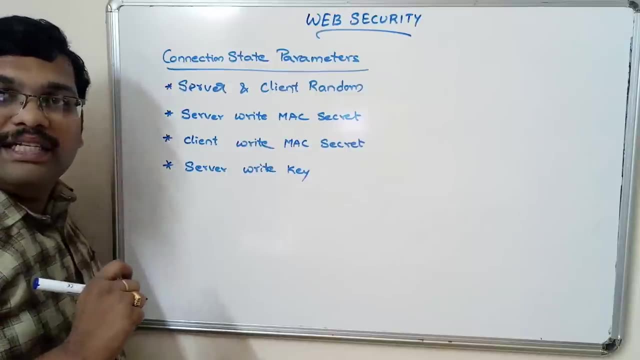 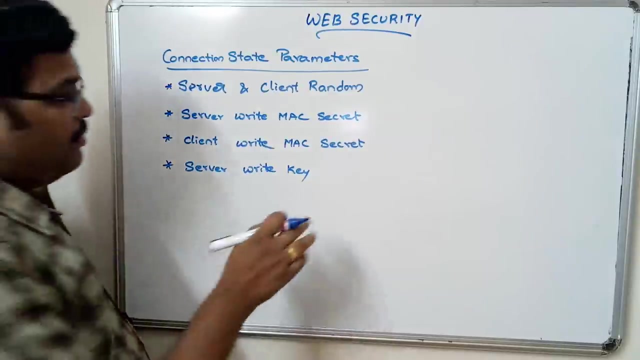 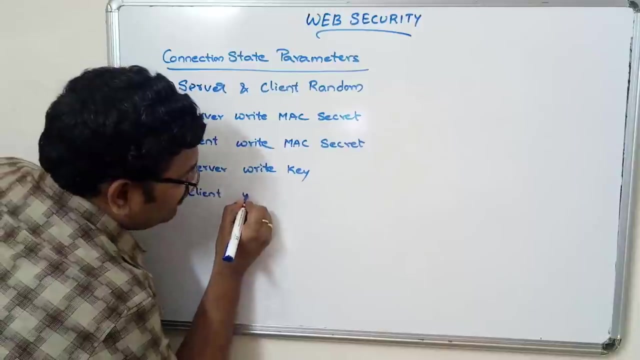 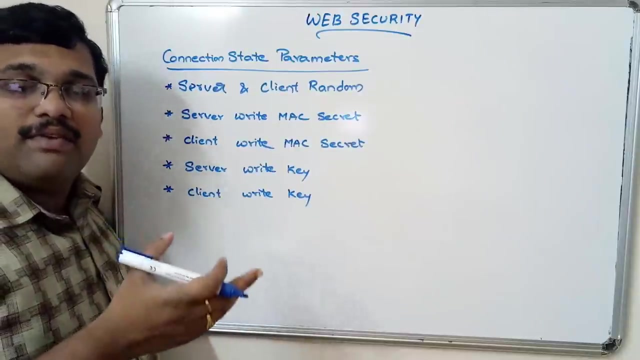 Server write key. So this is the MAC, the secret key used for conventional encryption. this is the secret key which is used for the conventional encryption by the server, which is sent by the server. the client right key. so this is also the shared key between the client and server, but this key is generated. 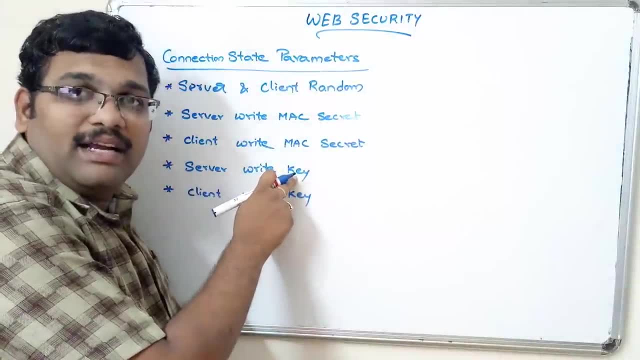 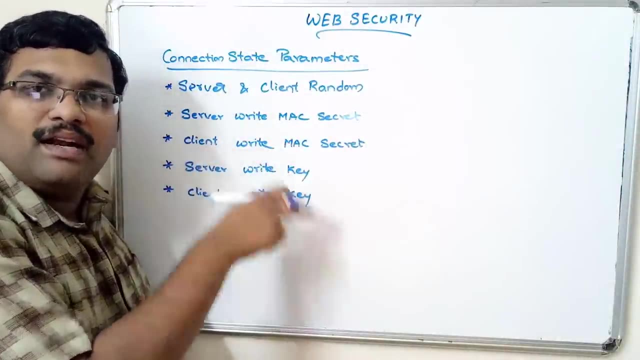 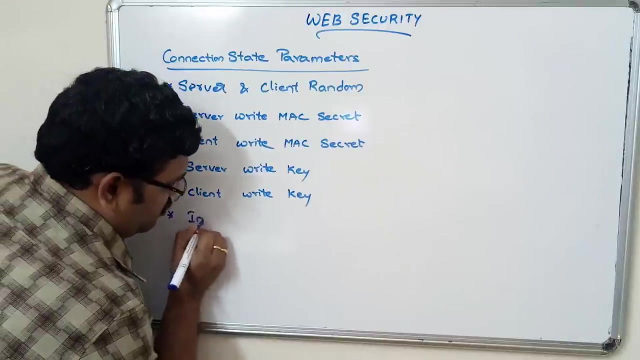 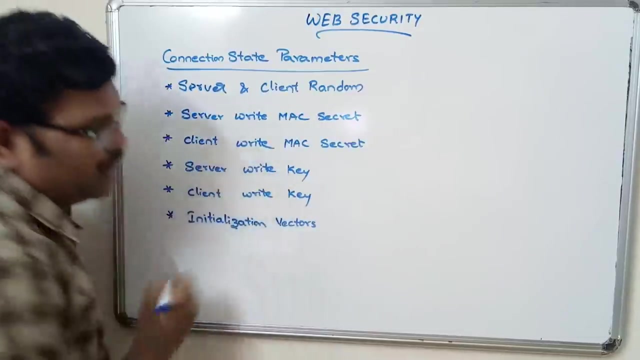 by the client. this key is a shared key, I mean the secret key which is shared among the client and server, but it is generated by server. so these keys are used for conventional encryption. next, initialization: we broke it initialization. let us not just like a buffer saw some dummy. 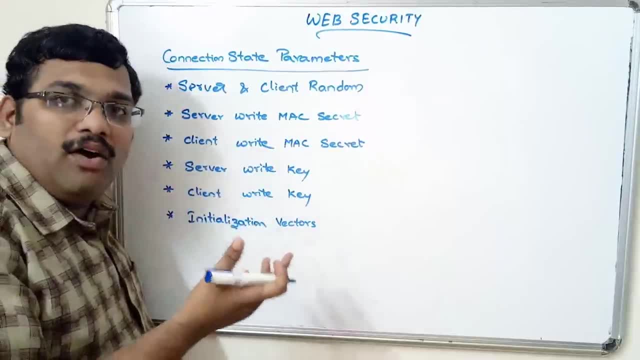 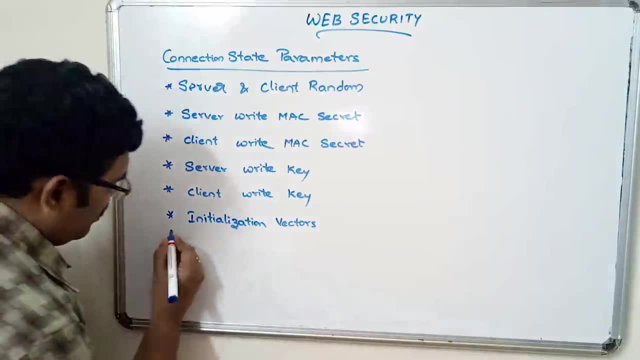 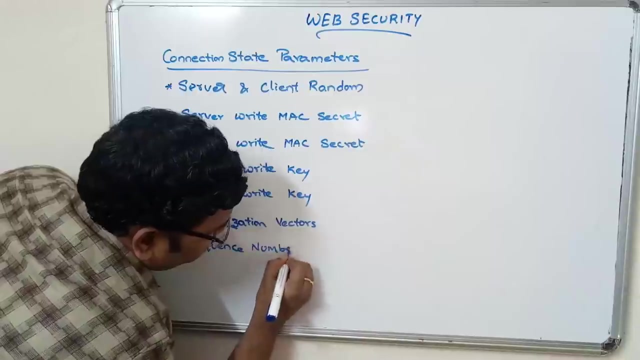 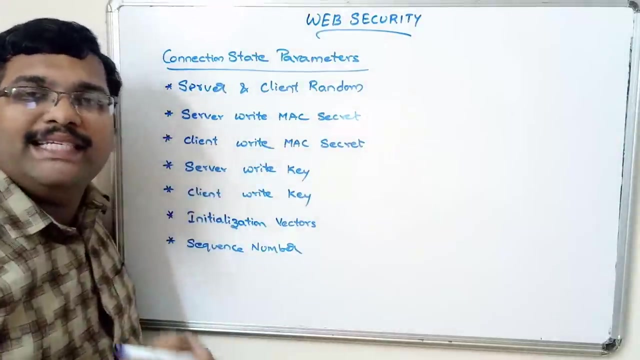 bits for the data or for the key in the mode of operation, the block cipher mode of operation. and the last one is sequence number. as you know, the sequence number will be generated and it will be appended to each and every packet which has been sent through the transmission. 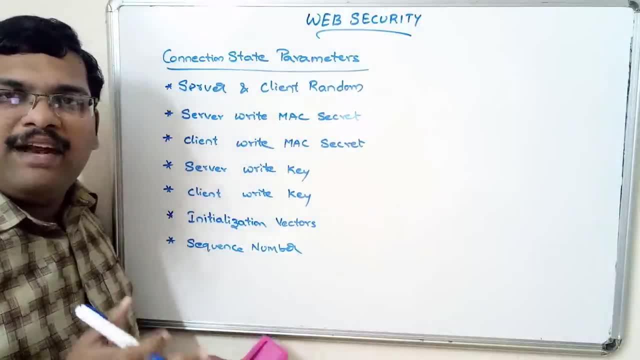 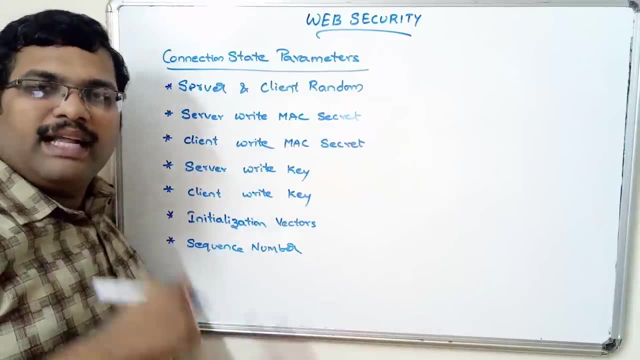 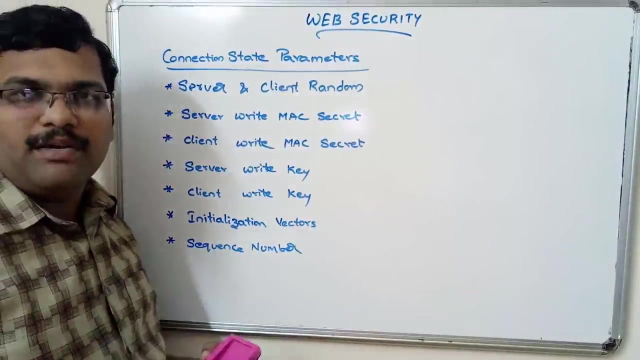 right during the transmission. so, based upon the bandwidth, the complete data will be fragmented and the sequence number will be allocated for each fragment and the receiver side, they will collect all the packets and they will collaborate all the packets according to the sequence number right. so these are the parameters associated with the connection. 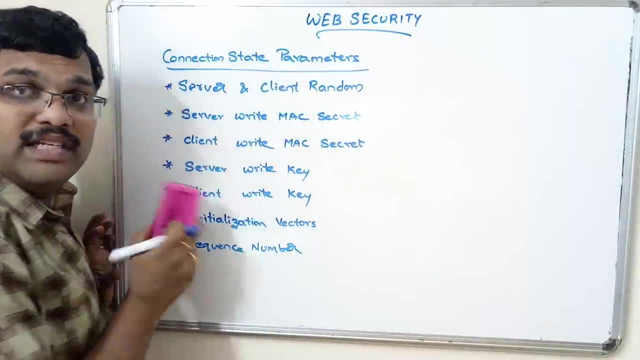 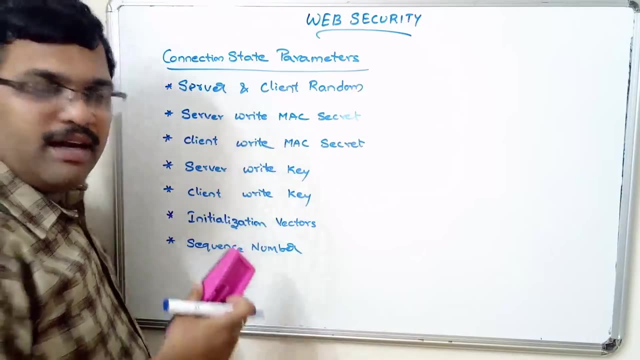 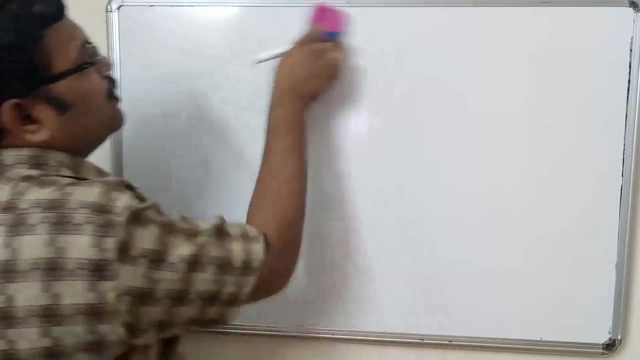 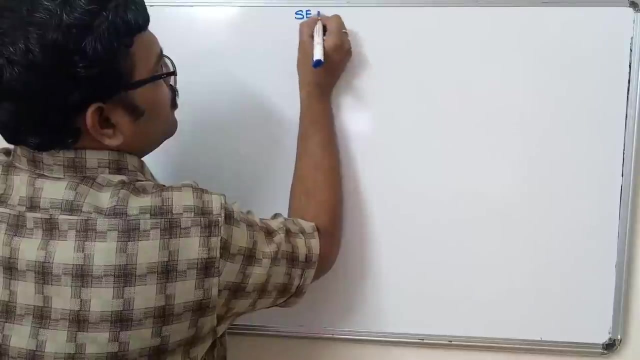 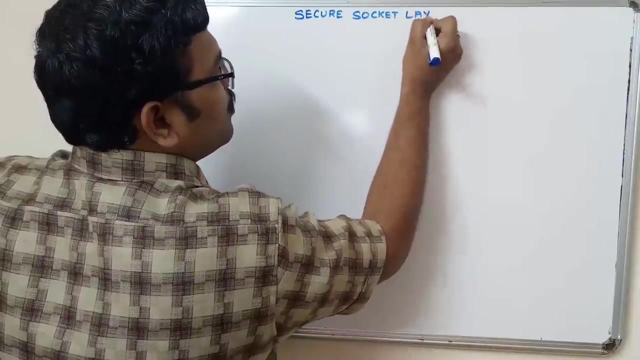 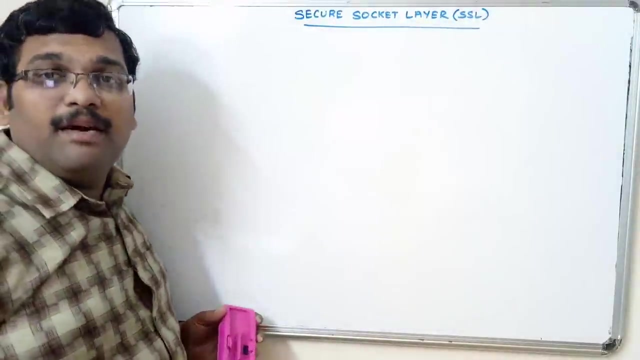 now hope you understood this session state parameters and the connection parameters. now let us move on to the SSL secure socket layer- secure socket layer, which we call it as SSL. so this is implemented by using the SSL protocol stack just above the TCP and just below the HTTP. 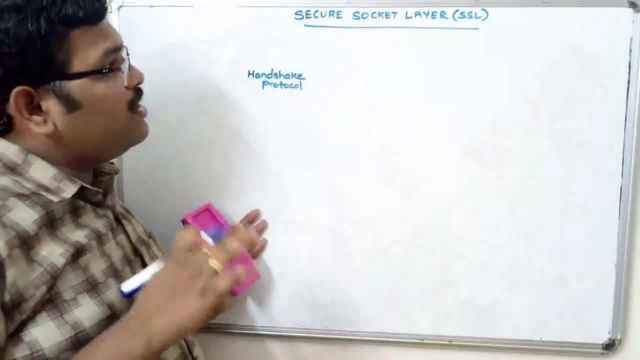 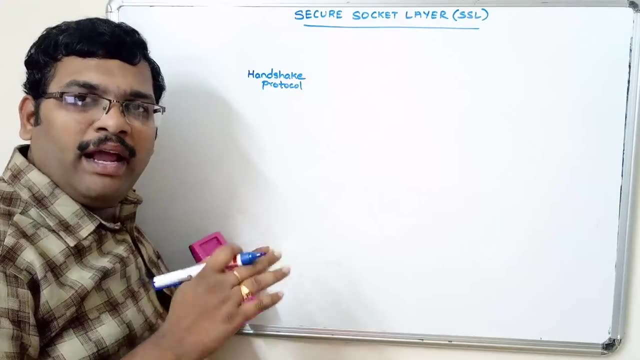 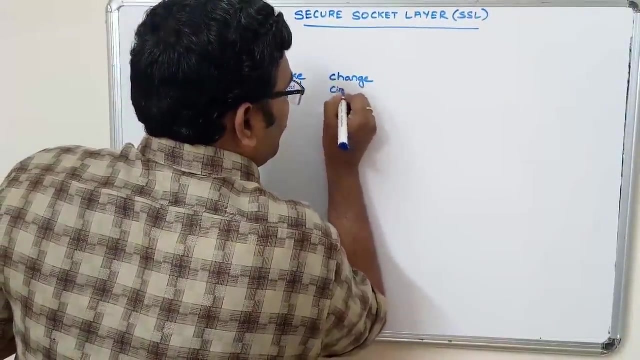 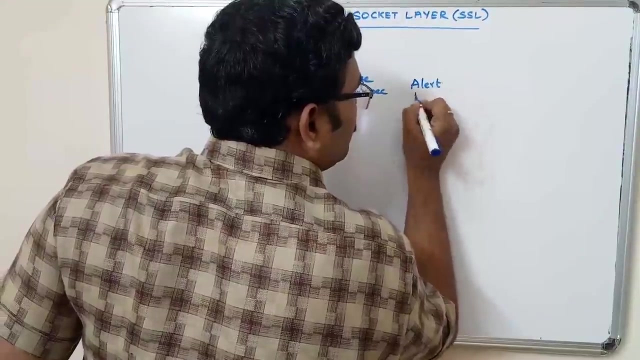 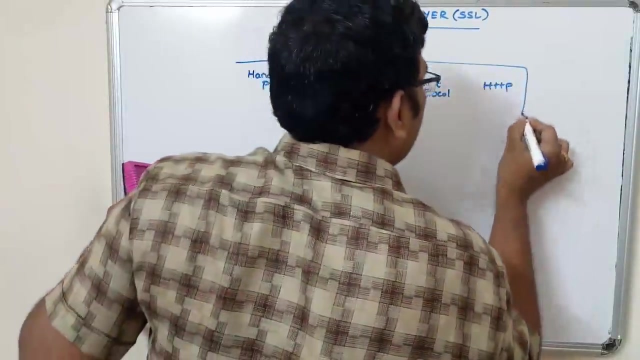 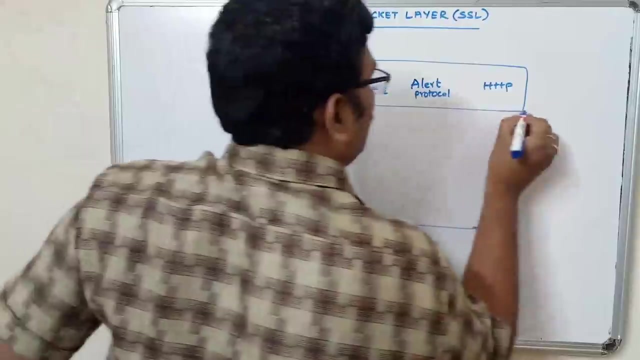 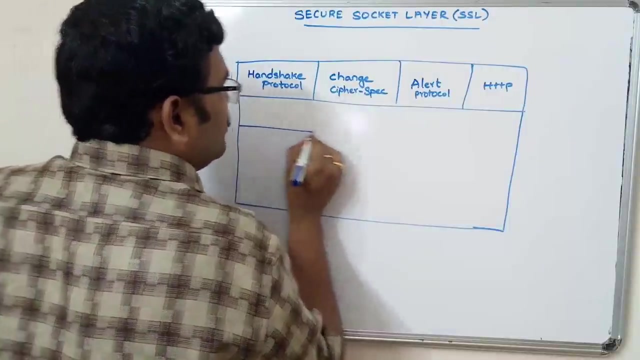 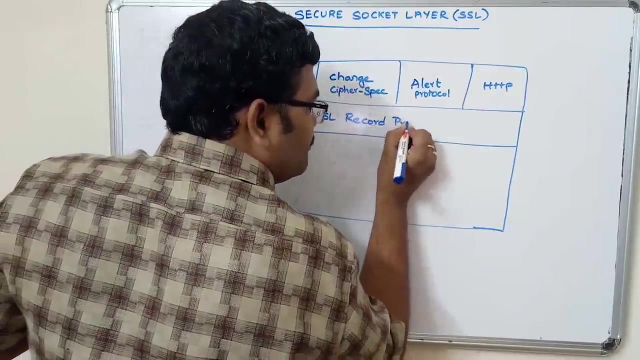 so, as we discussed earlier, this protocol stack will be having four protocols. one is SSL record protocol, handshake protocol chain, cipher spec protocol and the alert protocol chain. cipher spec protocol, alert protocol and finally the HTTP. the next one is SSL record protocol, where the data fragmented and the day the calculation was done correctly. 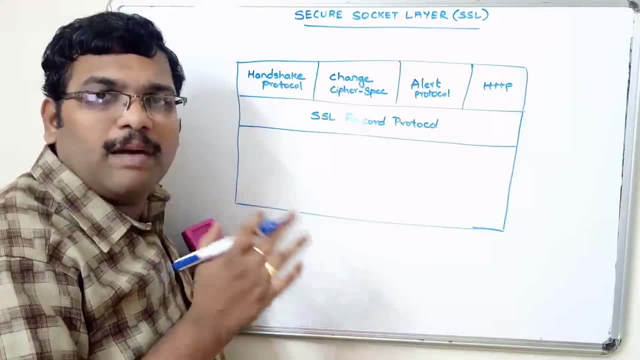 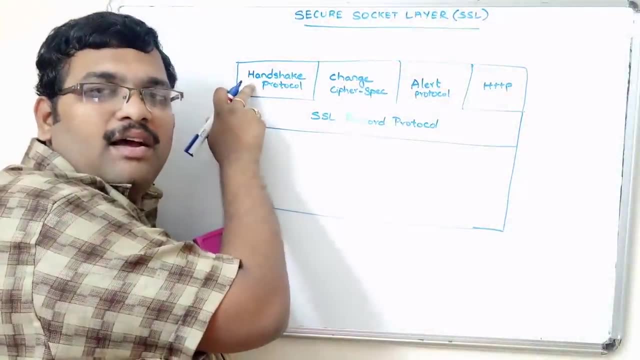 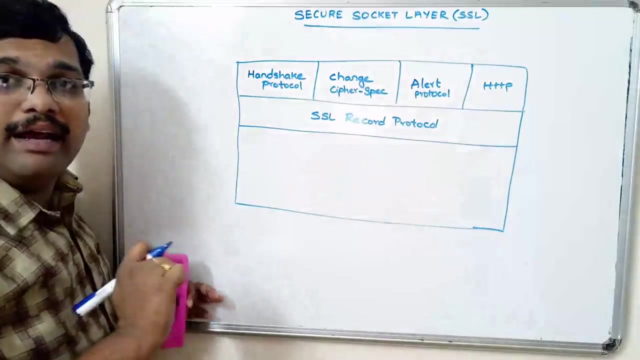 and the calculation of MAC or the encryption algorithms or the compression algorithms will be implemented in this protocol and this handshake protocol is used to establish the sessions and this mainly this handshake protocol is used to authenticate the client with the server and the server with the client and chain cipher spec protocol is for changing the state, the pending state, to the current state. 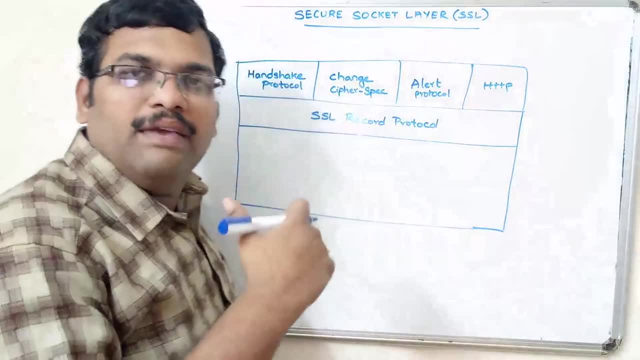 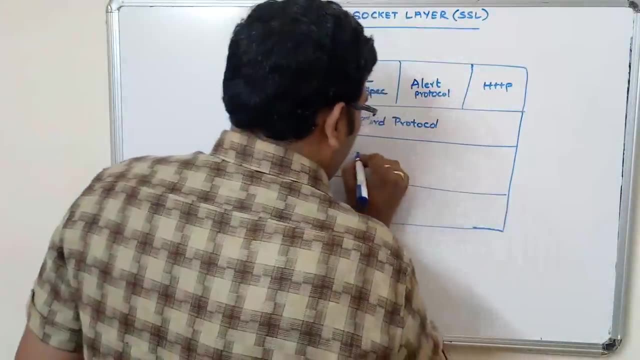 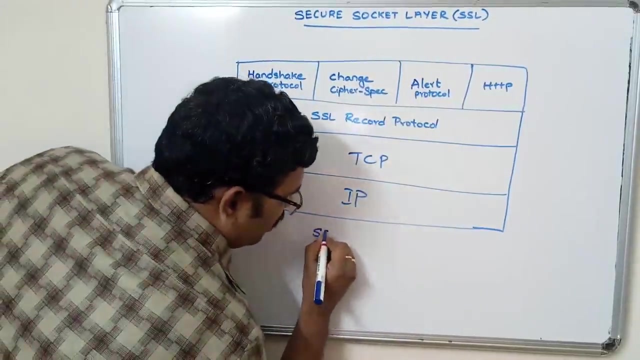 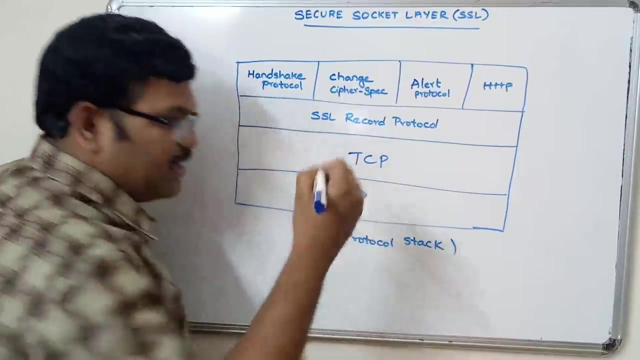 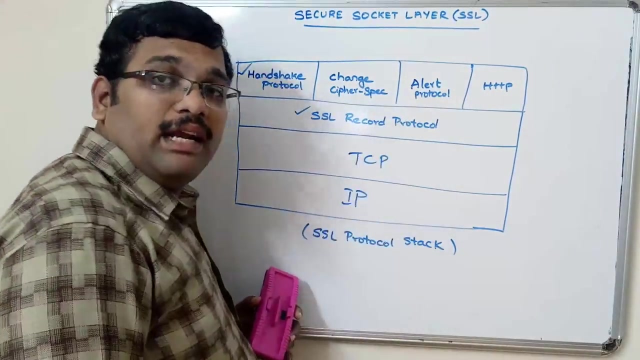 and this alert protocol for giving the alerts while implementing this SSL. these are, as usual. we know the TCP protocol and the IP protocol. so this is the SSL protocol stack- SSL protocol stack. so now let us look each protocol. first we will see the SSL record protocol, then we will move on to the handshake protocol. 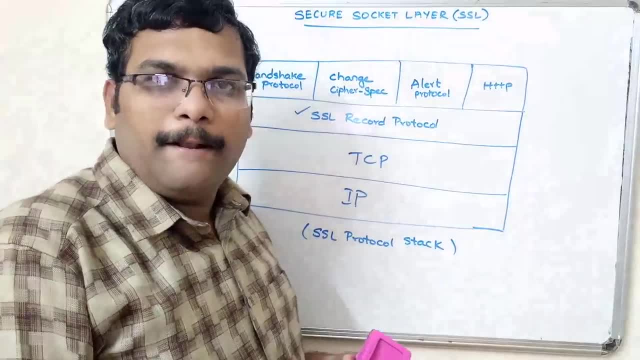 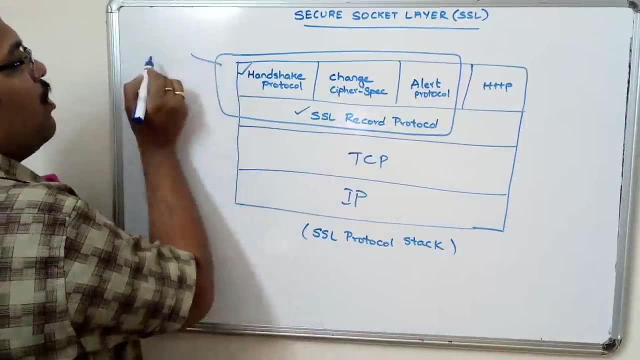 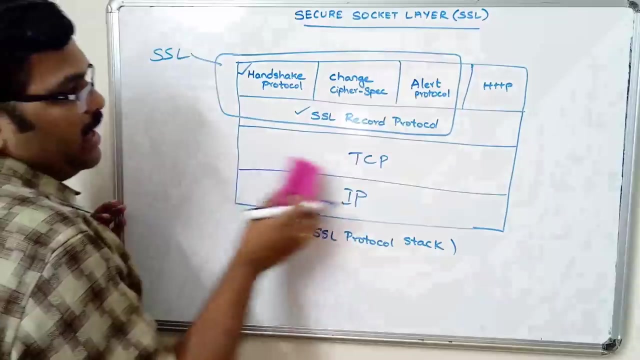 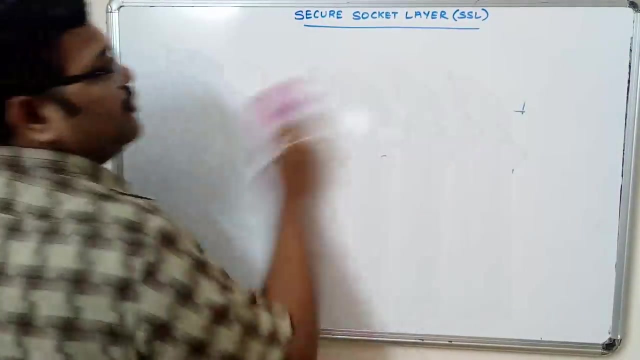 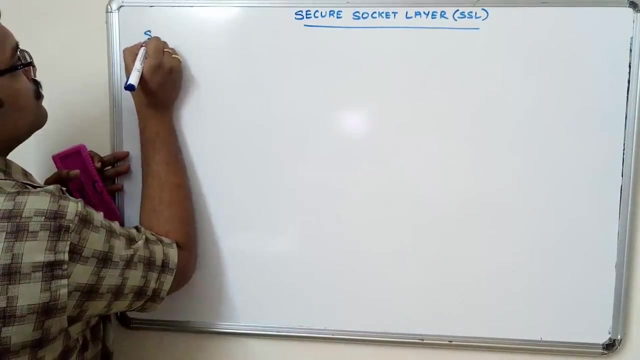 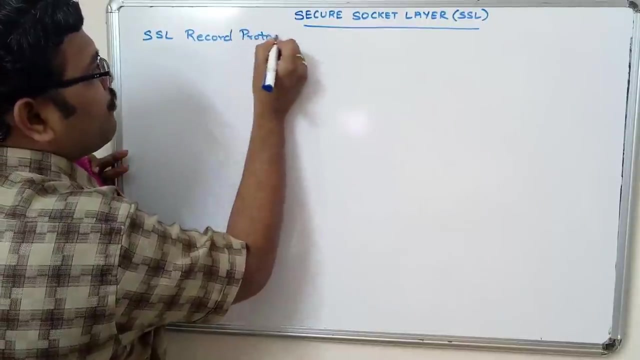 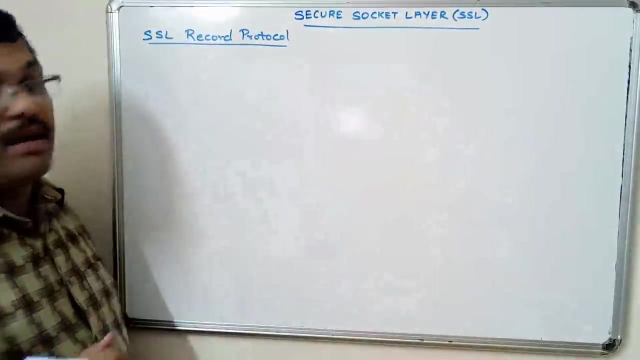 next, the chain cipher spec protocol and the alert protocol. so all these protocols, all these protocols are called SSL, involved in the SSL secure socket layer. now let us see the SSL record protocol, SSL record protocol. so here the actual implementation will be done. so the first step is the complete data will be taken. 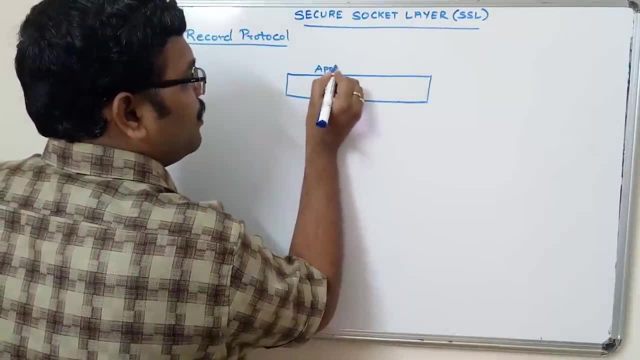 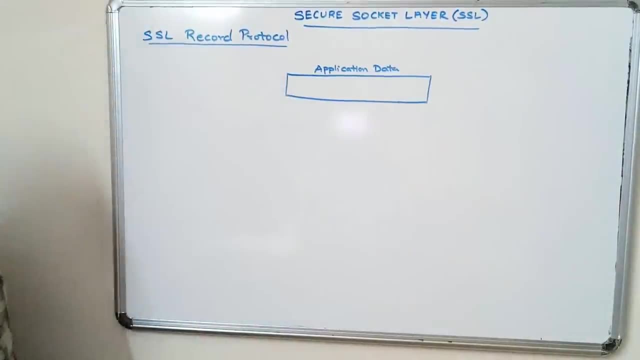 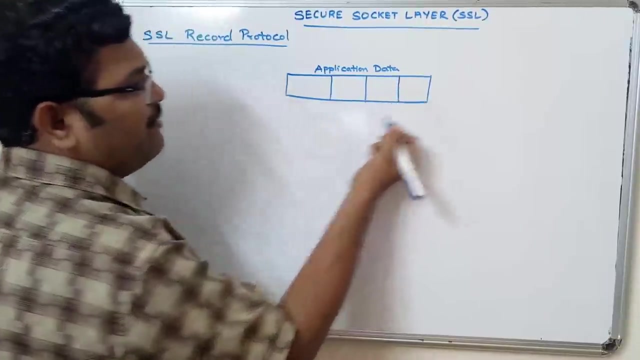 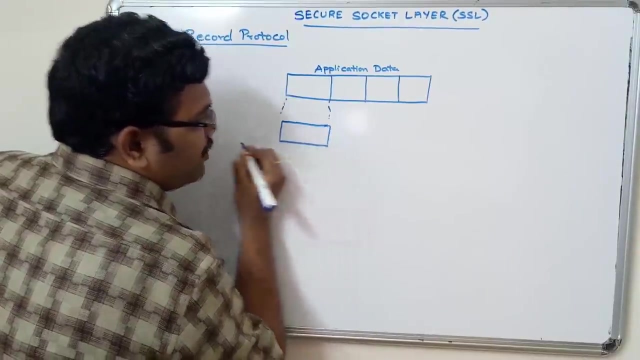 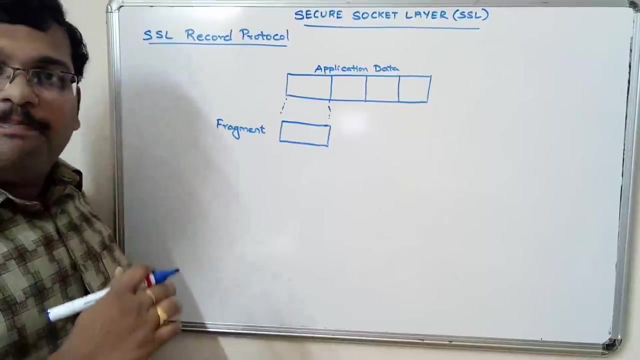 this is the application data, right? so this application data will be divided into different fragments. that means the fragmentation will be done according to the bank. so let us consider this fragment. so this is the fragment. so for each fragment we have to implement everything. so let us see the one fragment. 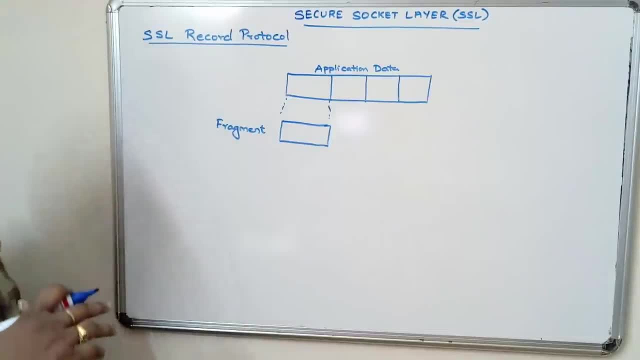 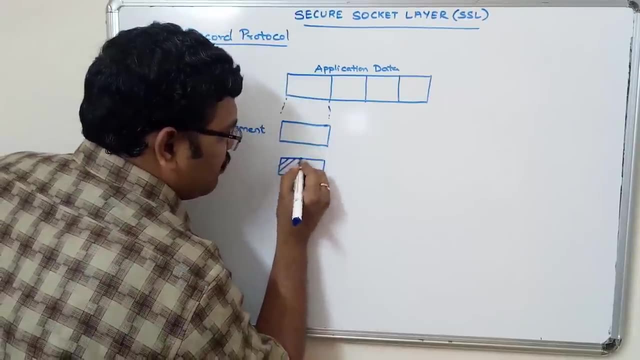 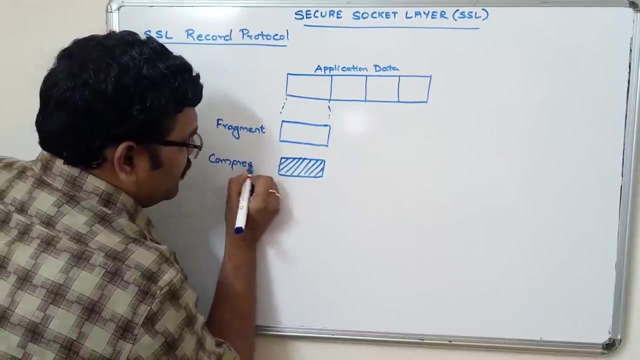 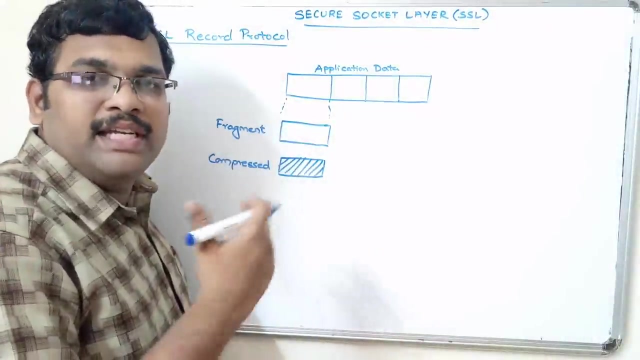 so consider the first fragment and now apply the compression function. so we have to apply the compression function. it is an optional thing, so apply the compression function. so the fragment in a compressed format. the fragment in a compressed format now calculate the MAC by using one of the authentication algorithm. 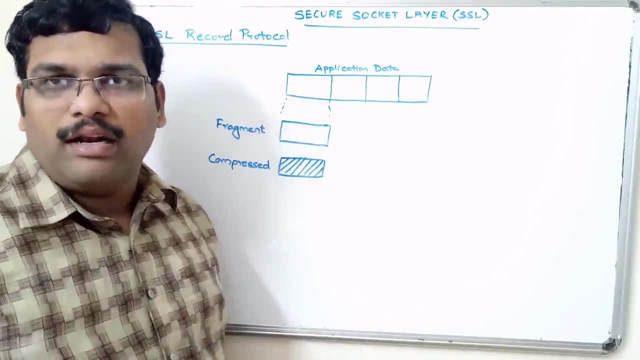 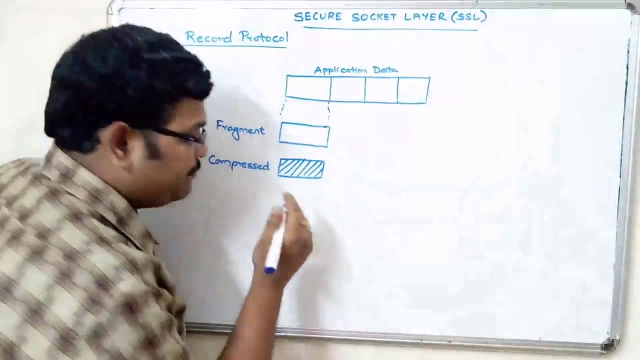 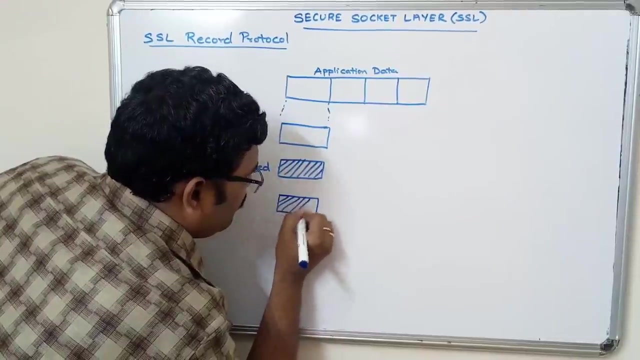 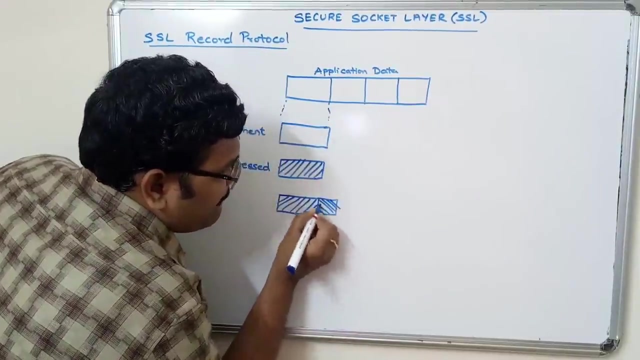 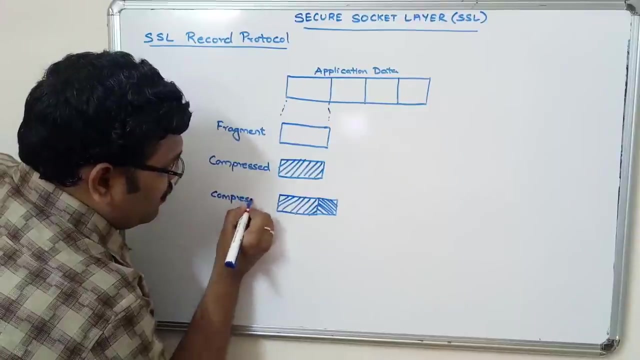 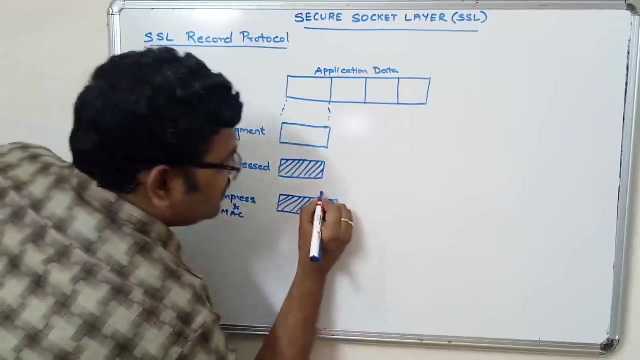 so here we can use the MD5 algorithm or a SHA-1 algorithm. so MAC will be calculated and the calculated MAC will be appended to the compression function. so this is the actual compression function and this is the MAC. right so, compressed function and MAC. so this is the MAC. 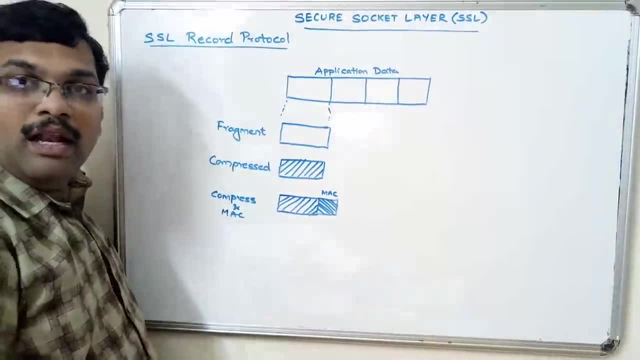 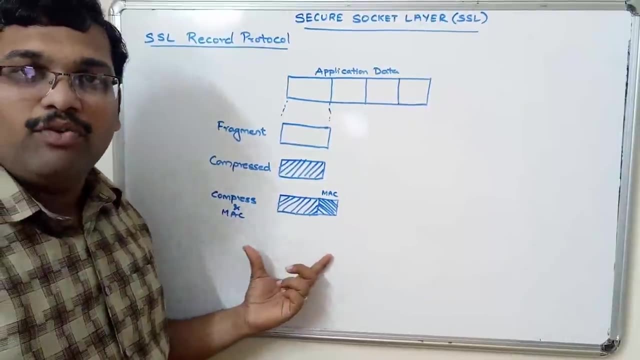 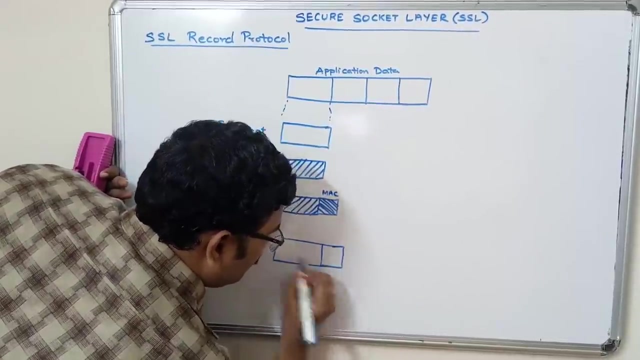 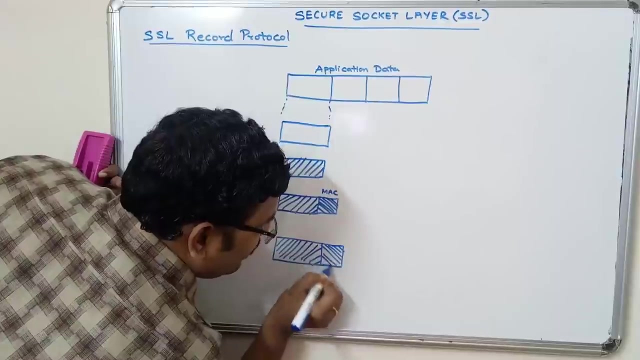 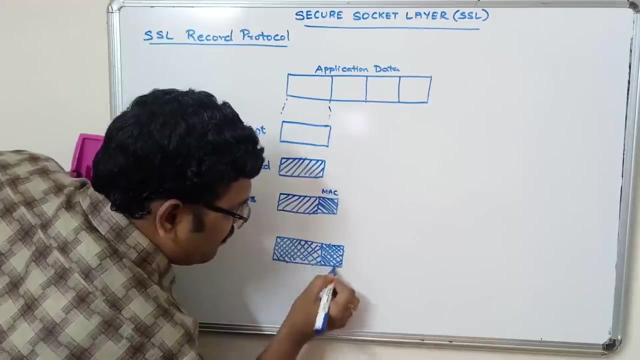 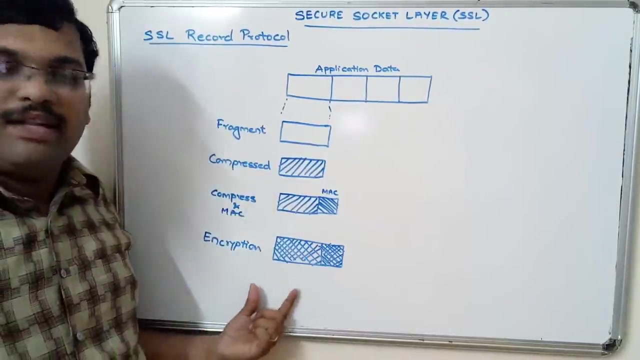 MAC which is generated for this compression function. now consider the complete compression function and the MAC. now we have to use the encryption, so we have to encrypt this data. see, this is the compression fragment, this is the MAC. now, encrypt this complete. now encryption is done, so encryption is done for this fragment. 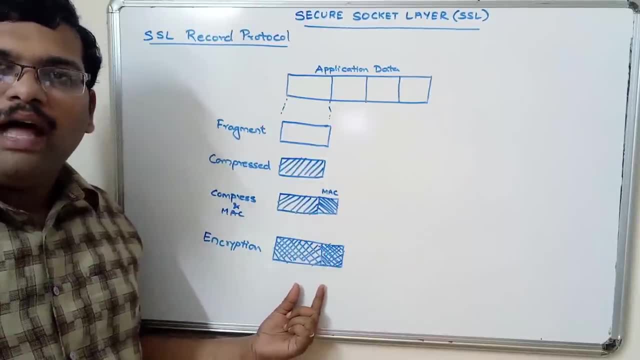 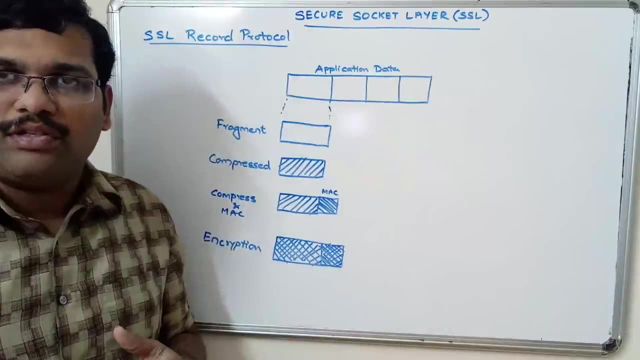 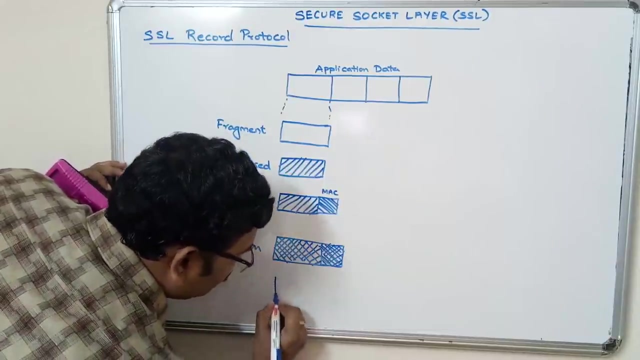 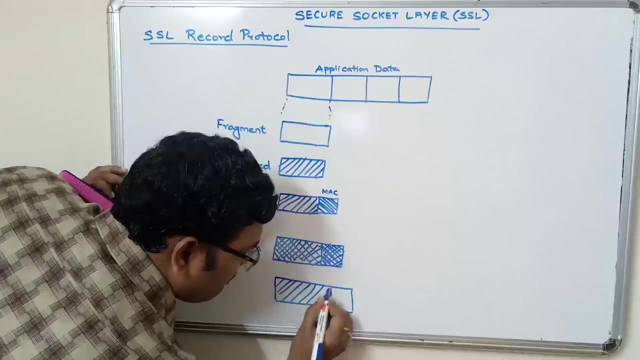 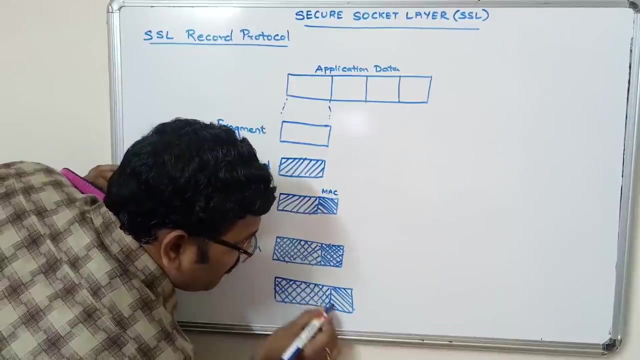 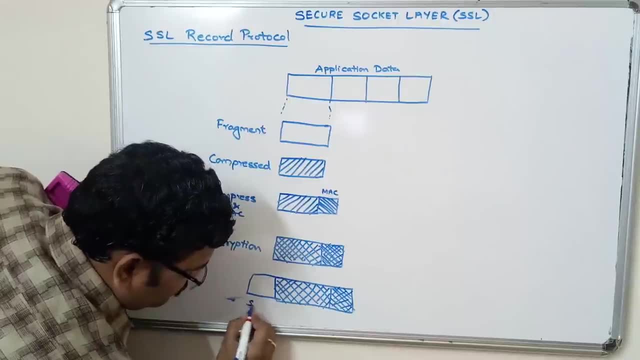 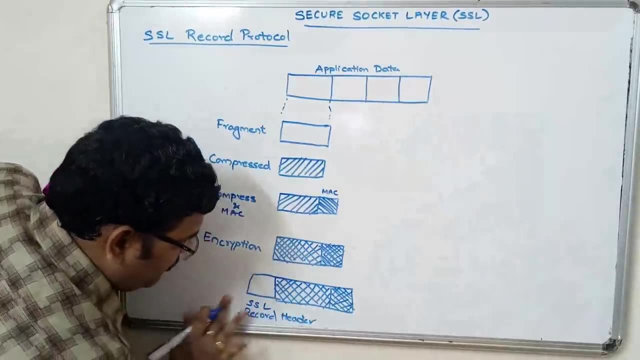 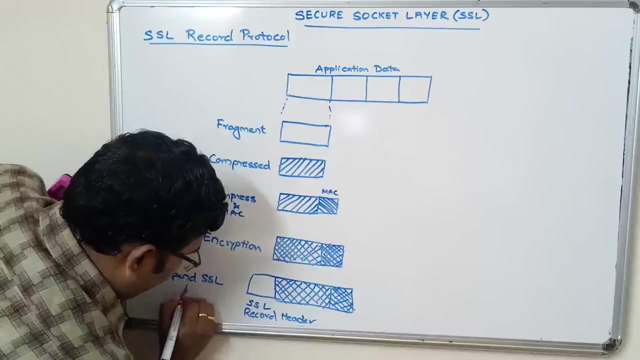 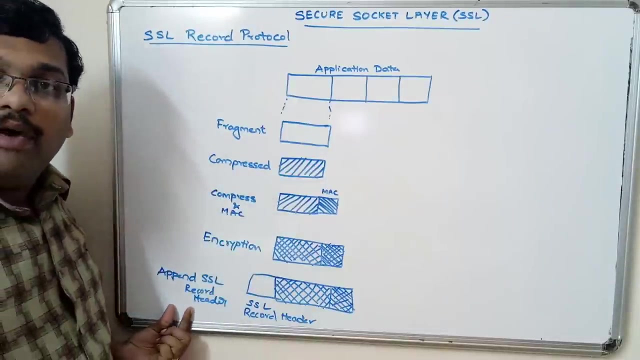 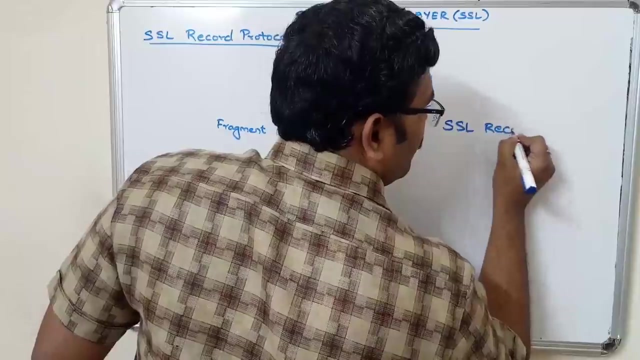 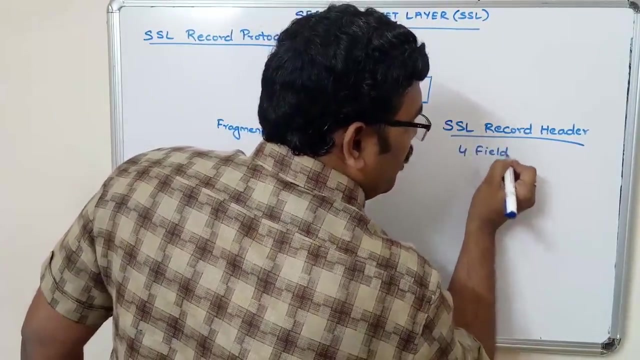 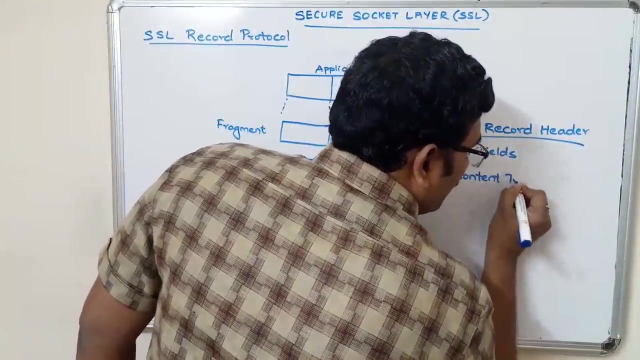 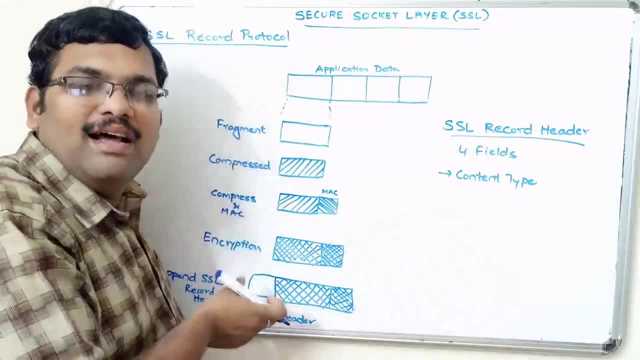 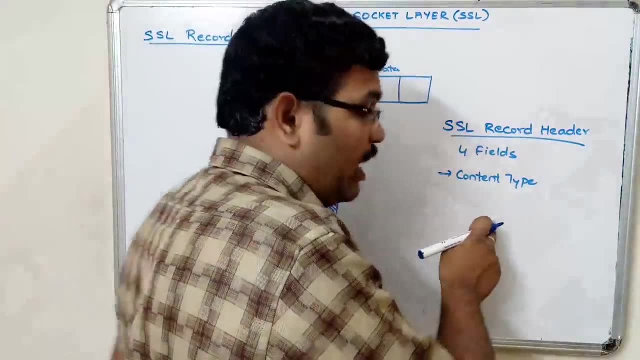 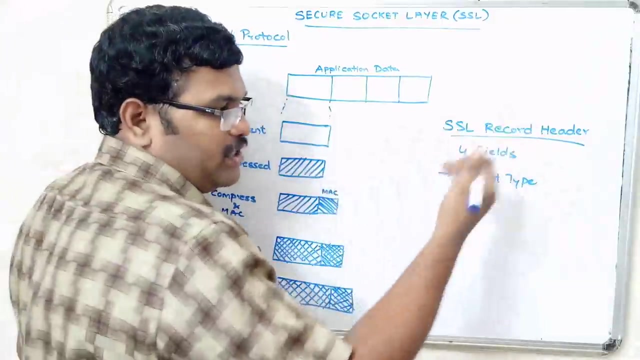 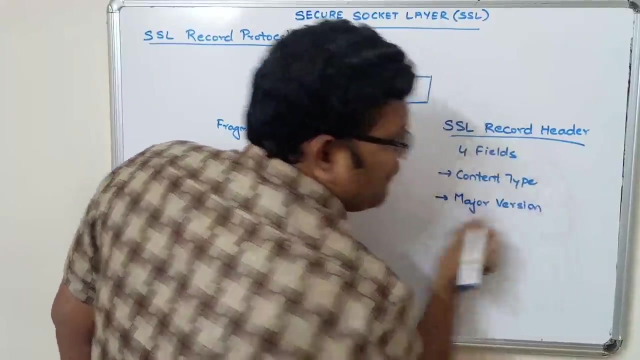 mention the higher layer protocol to which this compressed and encrypted fragment will be sent. So we have to implement, I mean, we have to include the higher layer protocol to which this fragment will be processed. And the next one is the major version of SSL. Major version of SSL. So here the major version of SSL is 3.. 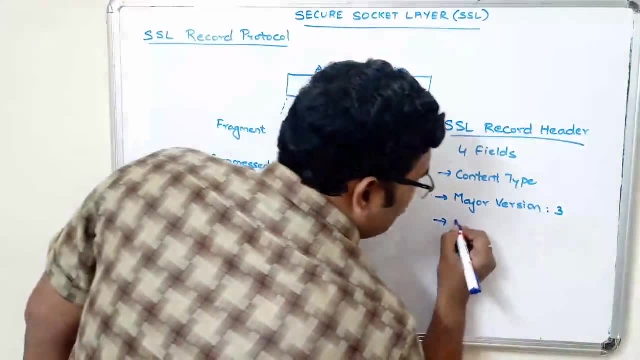 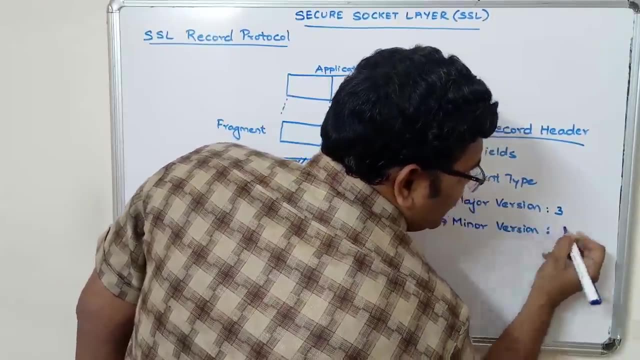 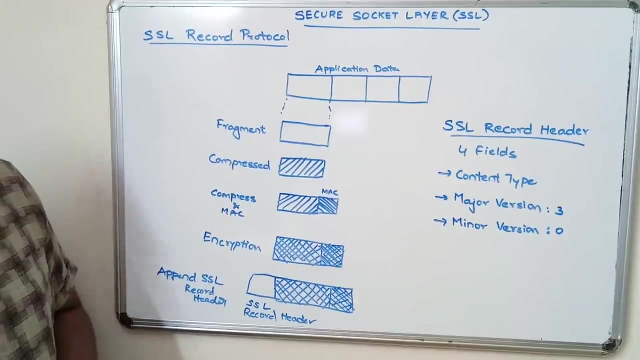 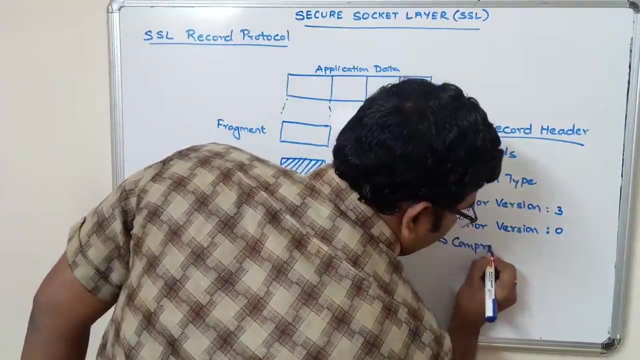 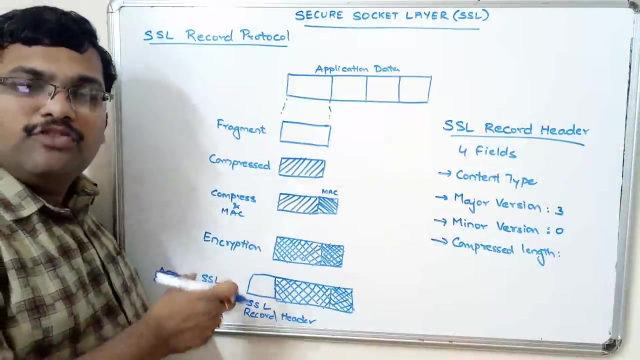 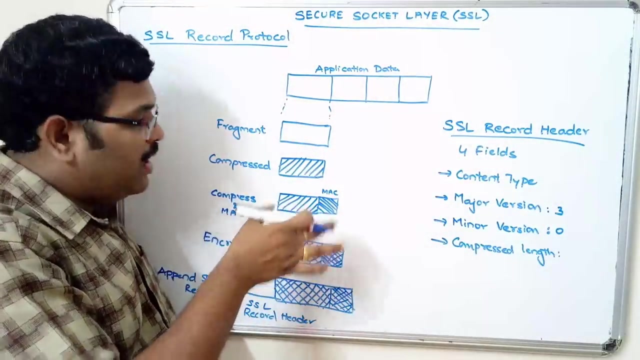 Right. The next field is minor version of SSL. The minor version of SSL, which is 0.. The minor version is 0.. Next, the last one is compressor length. So the length of the compressor length is 0. So this is the length of the compressor fragment. So if we use this compression function, we have to give the length of the compressor fragment. If you are not using this compression function, just we have to mention the length of the plain text. 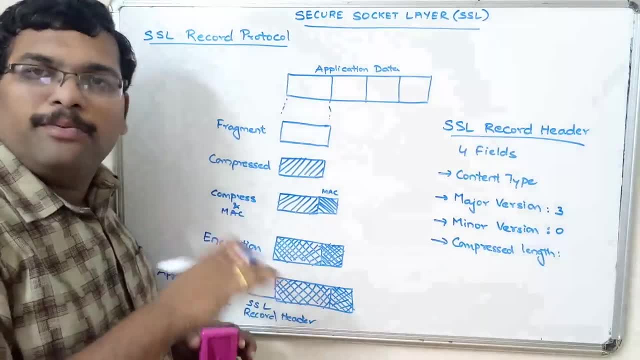 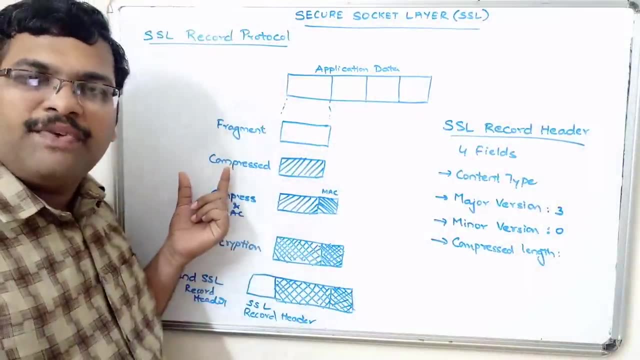 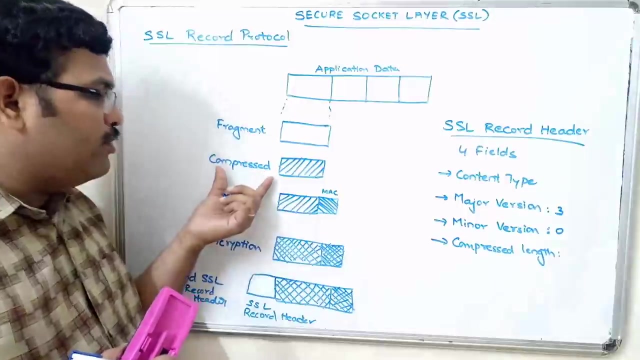 So hope you understood This. compression function is an optional thing. So here, if you want to include this compressor length, if we are using the compression function in our SSL, we have to give the length of the compression fragment. If you are not using any compression function in this SSL, we have to give the length of the plain text. 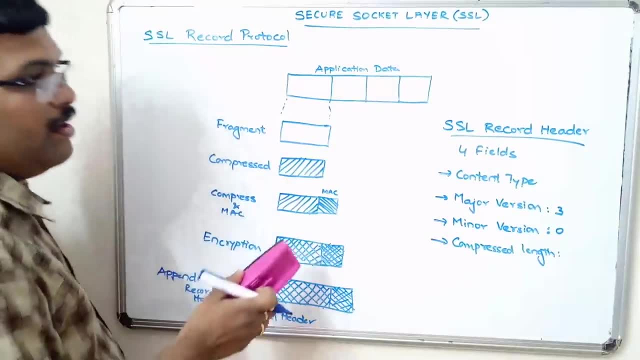 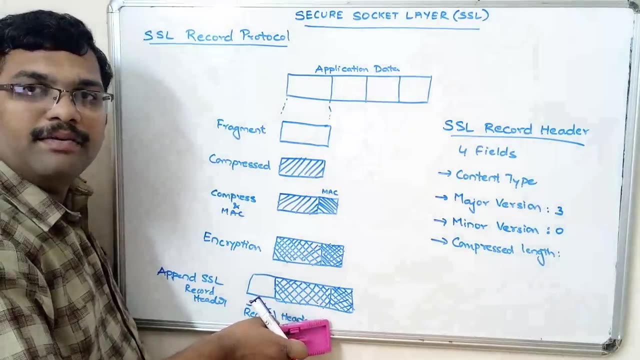 Right, These are the SSL record header, So this will be appended to the encryption fragment. Now, after applying all these things, how the record format will be. We will see how the record format will be. Let us see Now, after applying all these things, how the record format will be. We will see how the record format will be. Let us see. 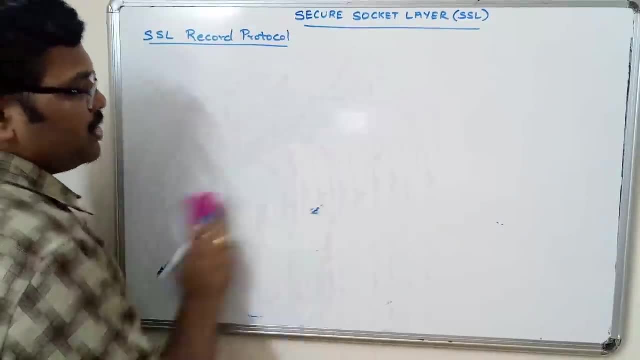 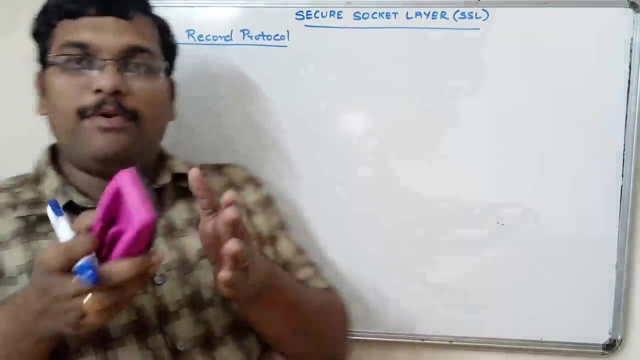 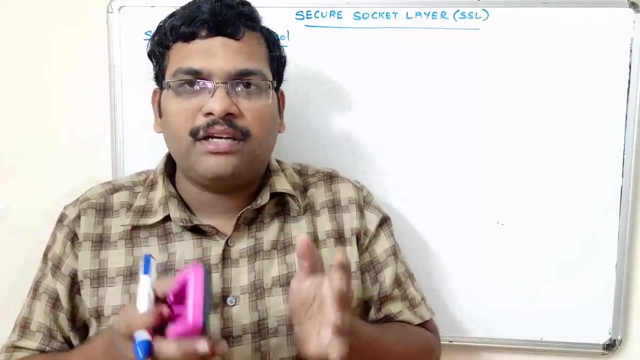 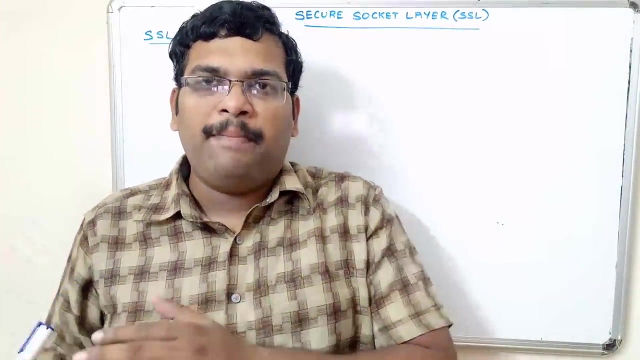 So, step by step, we are processing the fragment. 1st, consider the data, The application data. We call it as the application data. So, based upon the bandwidth, the application data will be divided into different fragments. So consider each fragment. Apply the compression function. After applying the compression function, generate the MAC using either MD five or SHA algorithm. So append the MAC to the compression fragment. 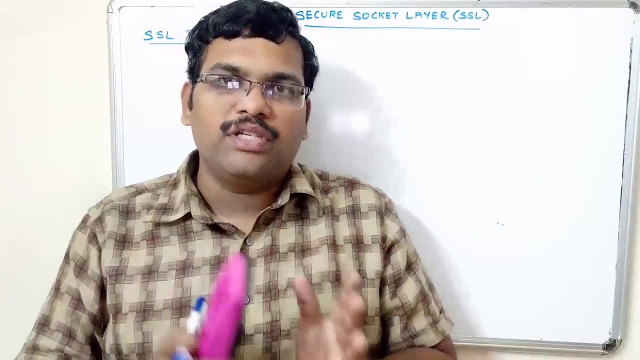 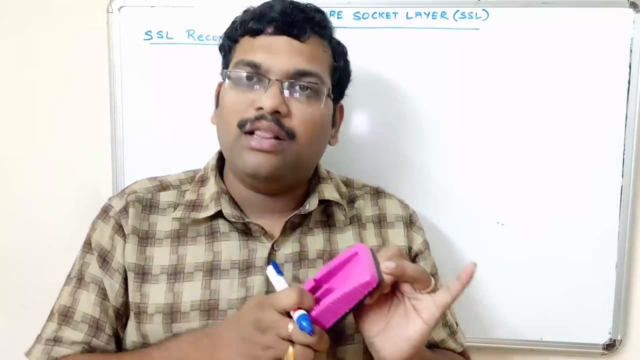 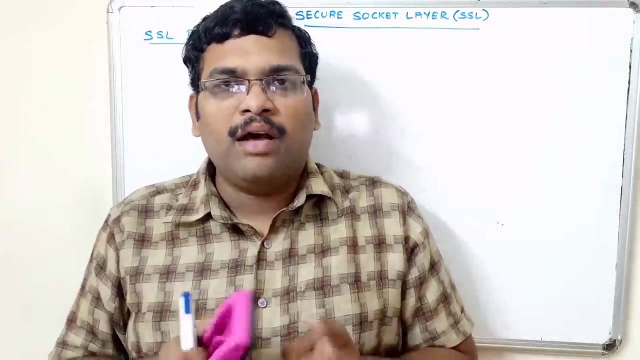 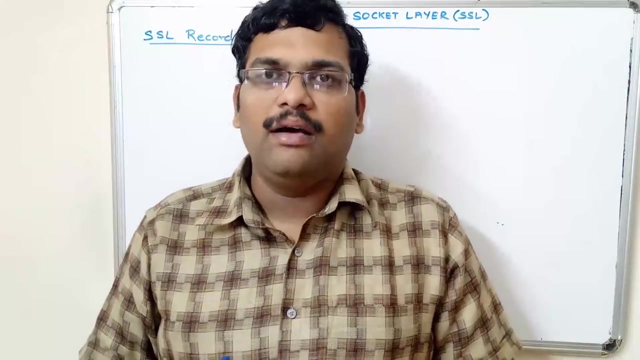 Now apply the encryption algorithm. So we can use either DES algorithm or IDEA algorithm or a triple DES algorithm- any algorithm we have to use. so by using all these- one among these algorithms- we have to encrypt the compressed fragment and, after applying the encryption, now append the SSL record header to that particular encryption and process the fragment to the higher layer protocols. 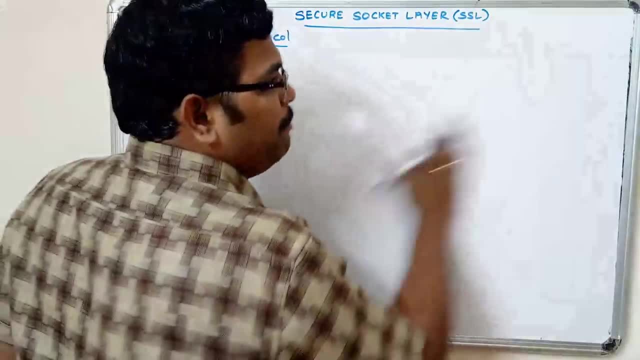 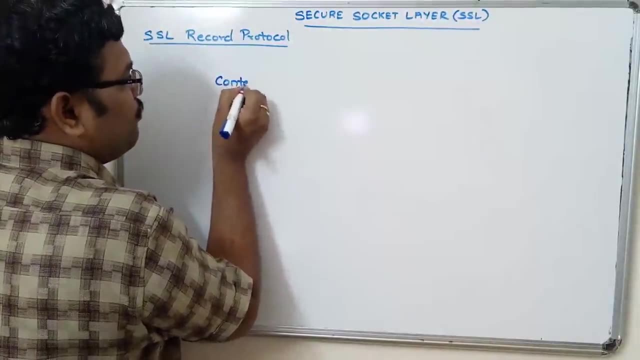 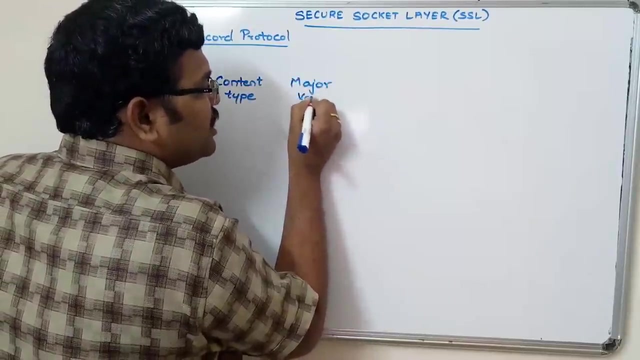 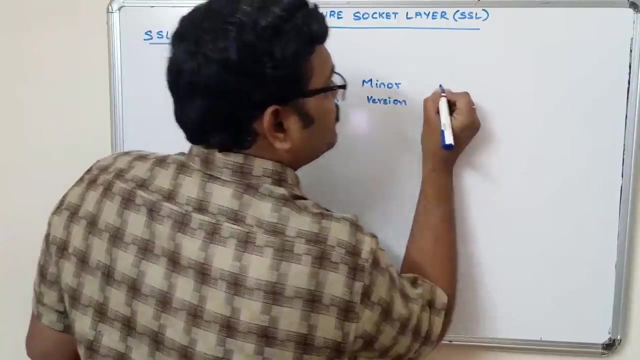 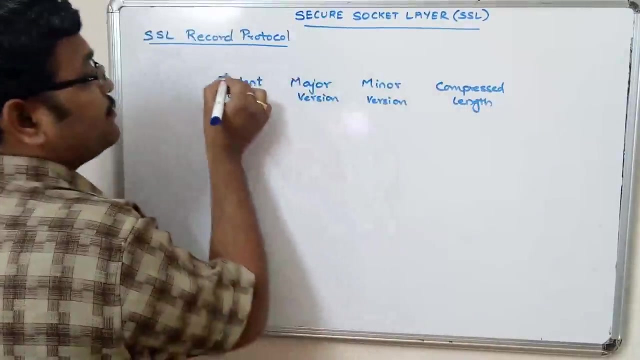 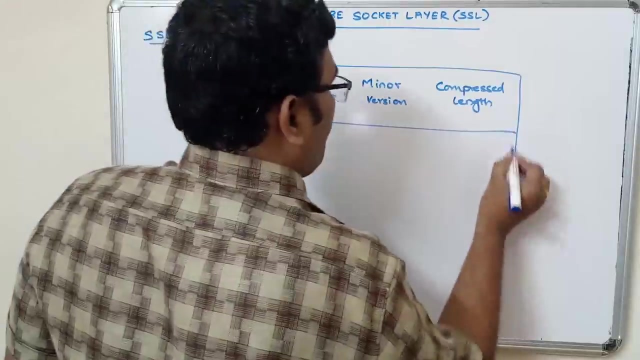 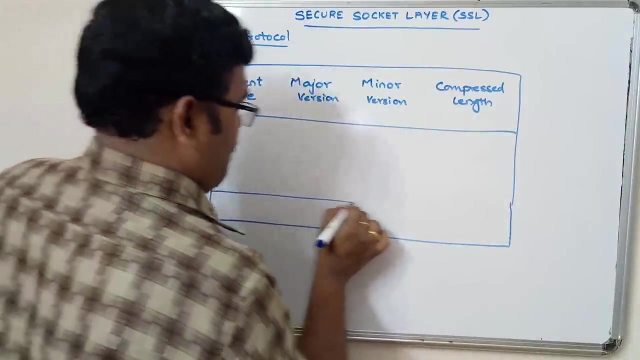 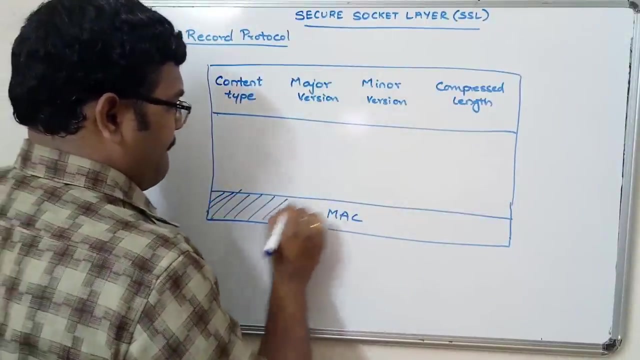 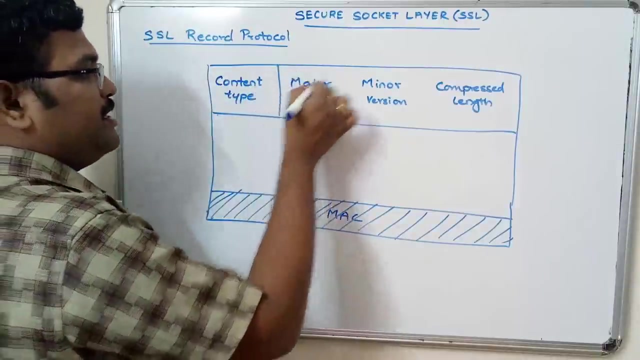 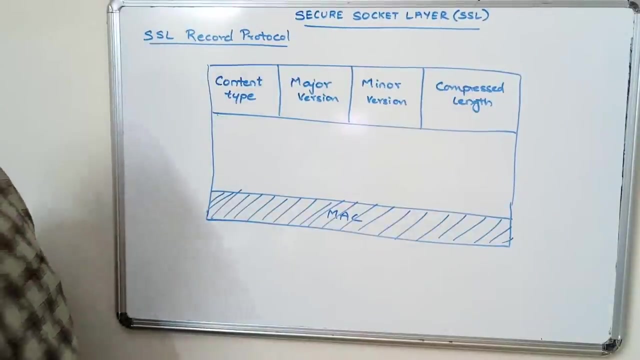 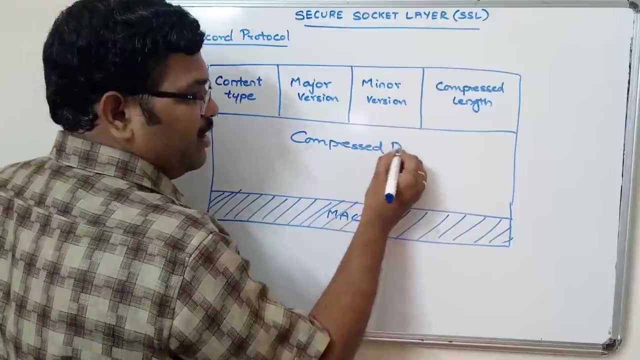 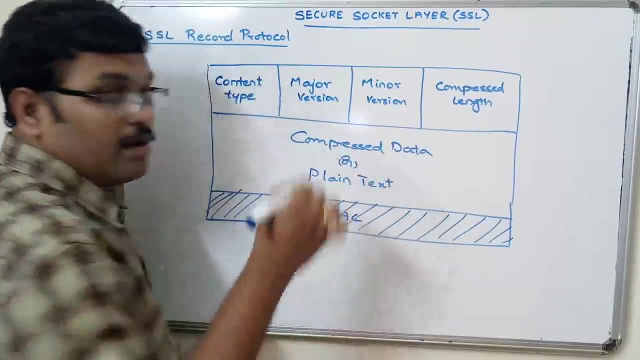 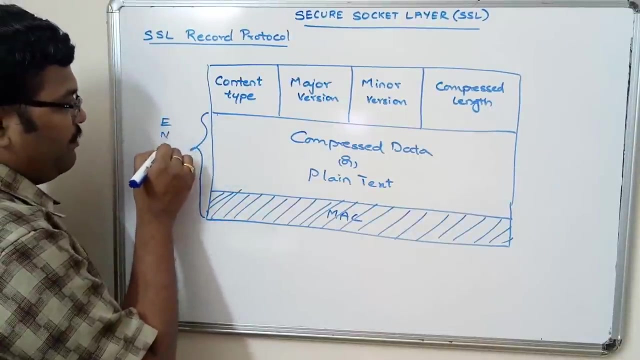 so let us see the complete output of SSL record header. the content type: major version, minor version, compressed length. this is the. this is the. this is the neck. this is the. This is the SSN record header. This is the compressed data, or it's a plain text. So here everything will be in encrypted format. 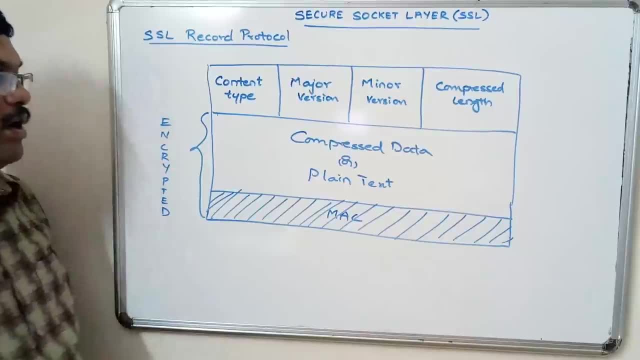 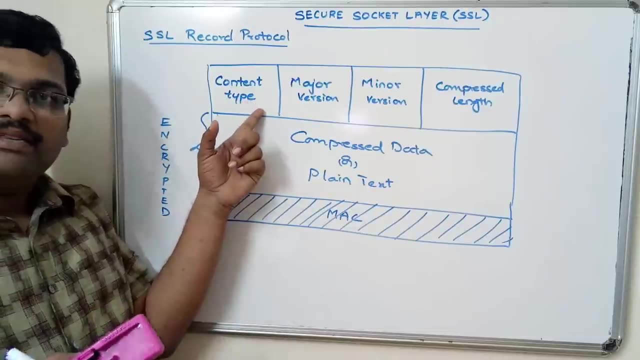 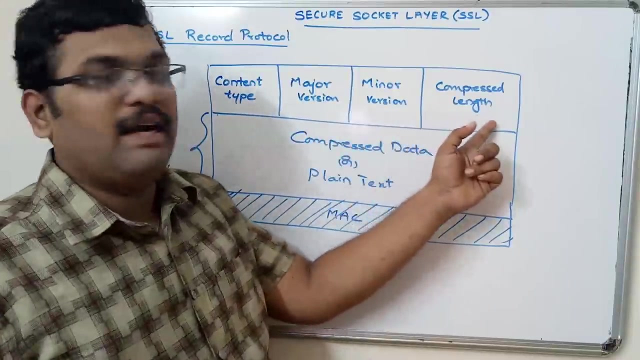 So all these things will be in a encrypted format. So this says the higher layer protocol to which this fragment will be processed. Major version is 3,. minor version is 0. and the compressed length: the length of the plain text or the compressed message. 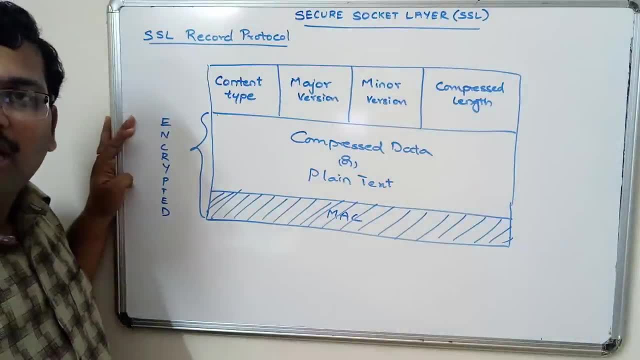 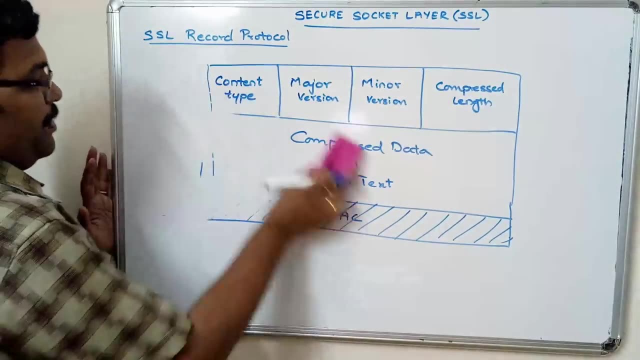 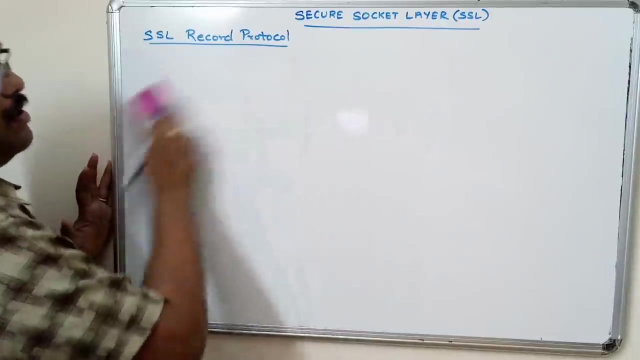 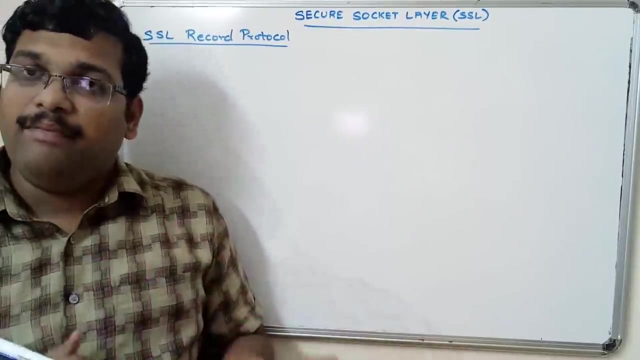 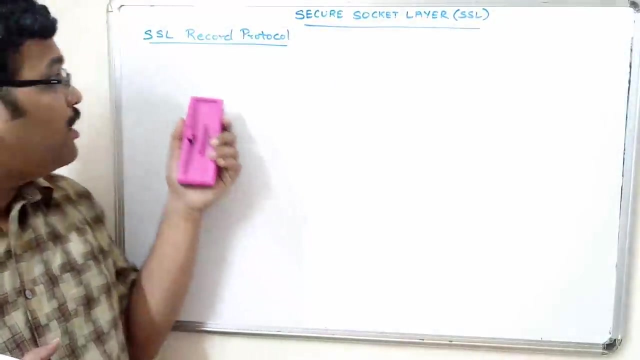 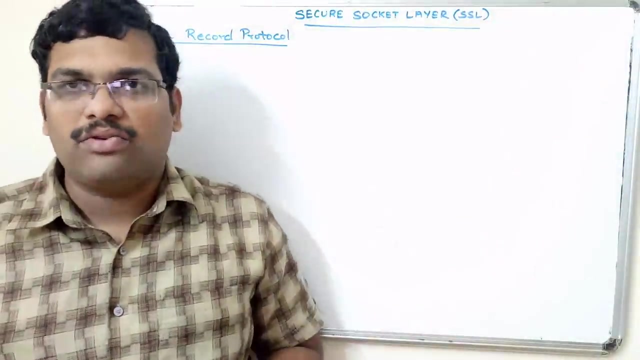 So this is complete SSN record protocol. Now let us see the calculation of MAC. So here the MAC is calculated by using either MD5 algorithm or the SHA algorithm. and the encryption algorithm, encryption process we are going, we are performing in this SSN record protocol is: we can apply either DES algorithm or triple DES or SSN record protocol. 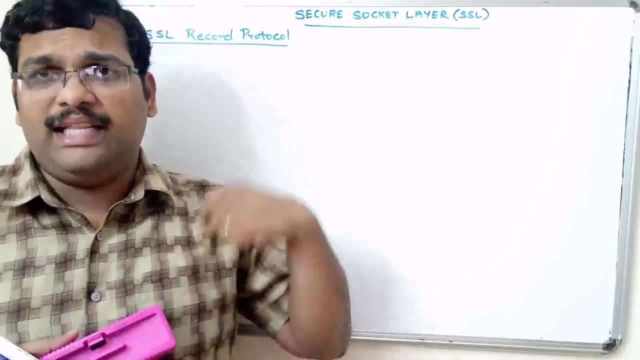 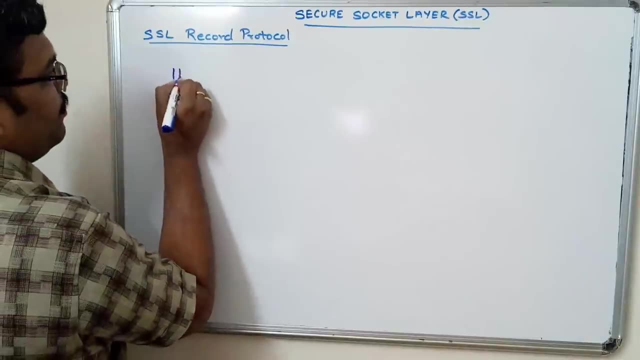 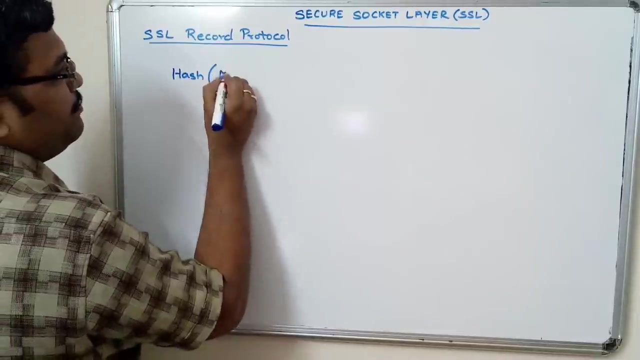 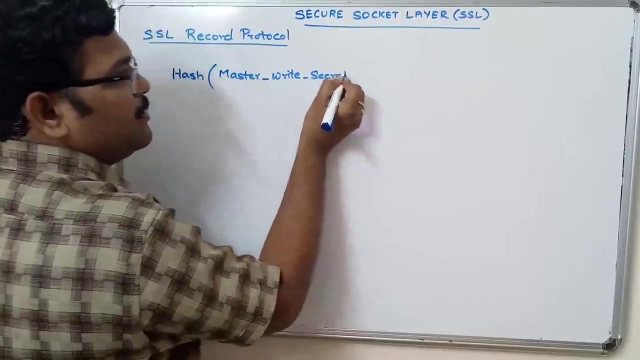 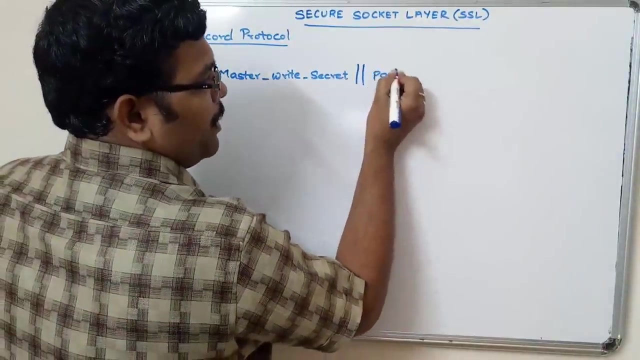 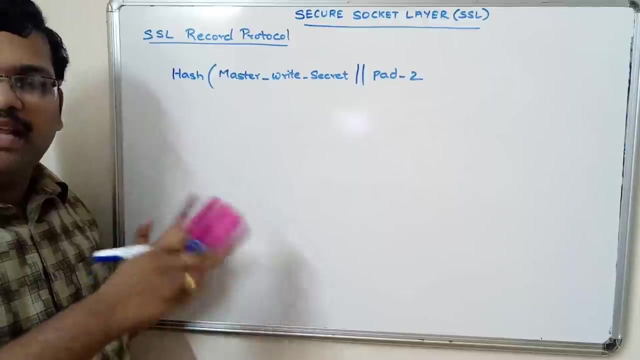 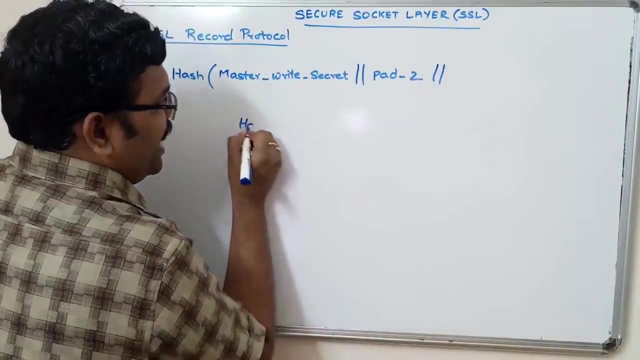 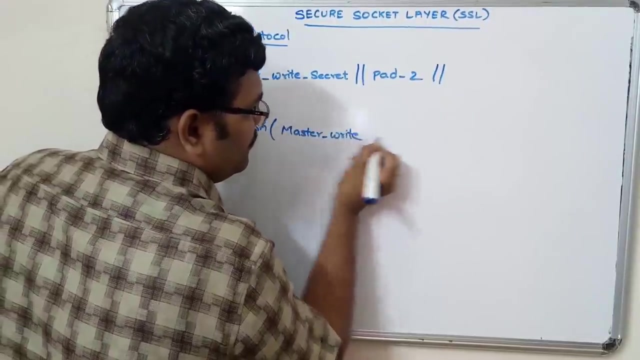 Any other encryption algorithm. Now let us see the equation for calculating the MAC. So let's see the error. Let's say we have pad 2.. I mean once I will write the formula first and then I will explain one by one. Pad 2, appended with again: apply the hash Master, write secret. 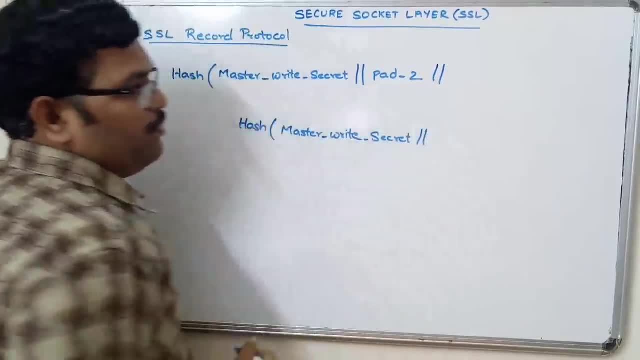 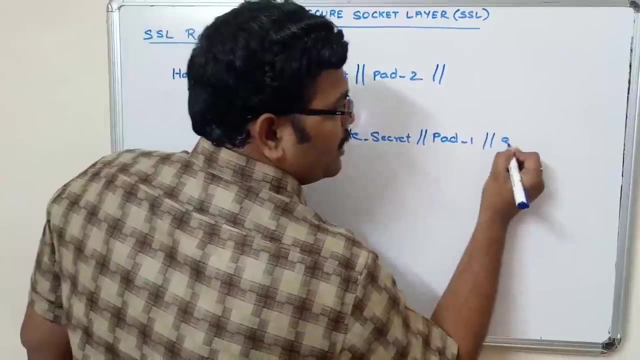 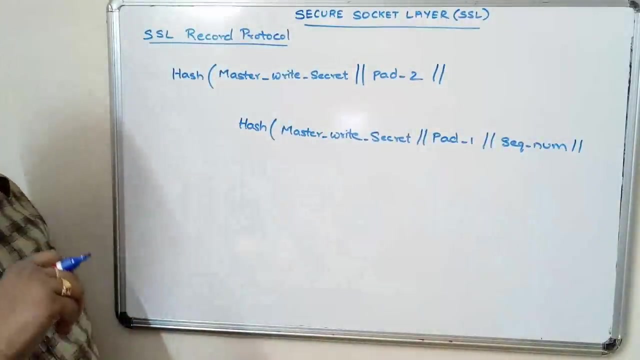 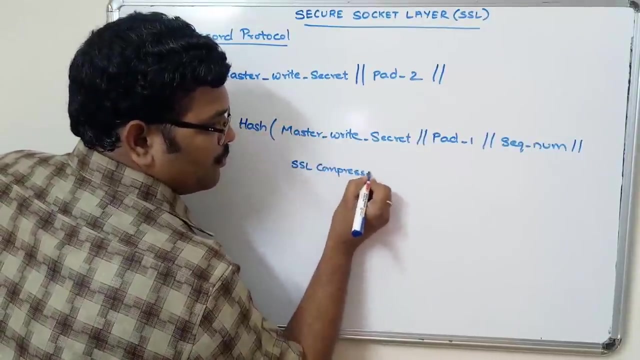 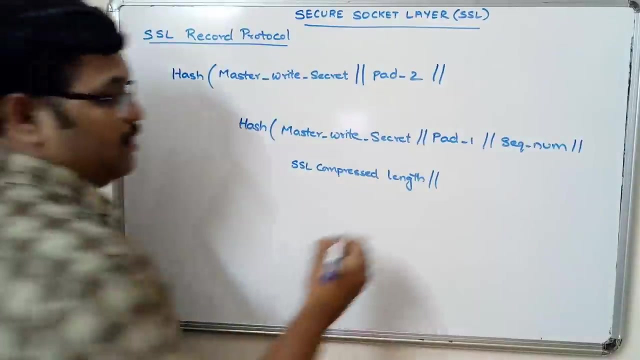 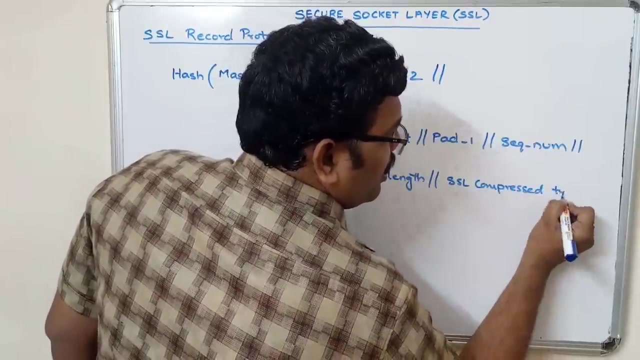 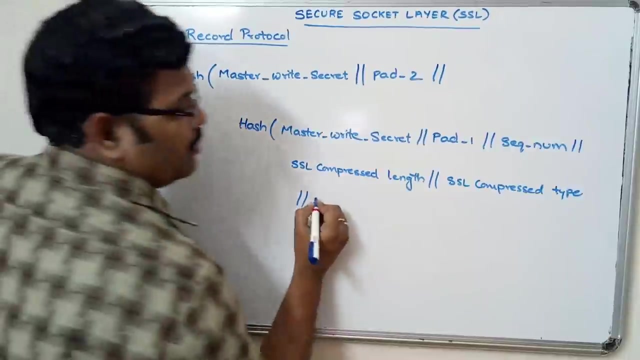 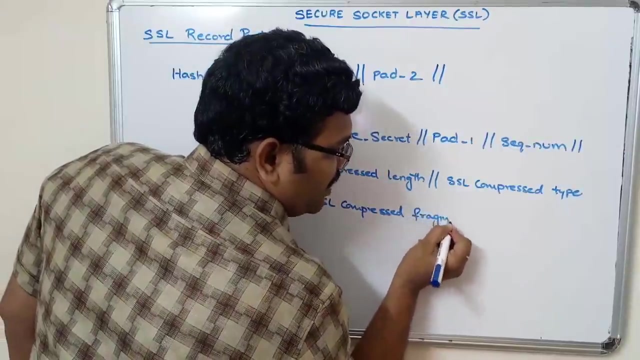 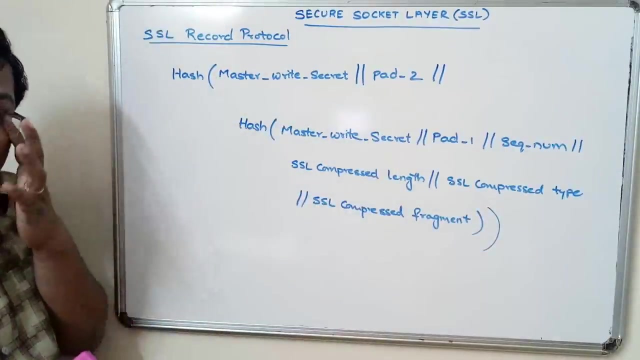 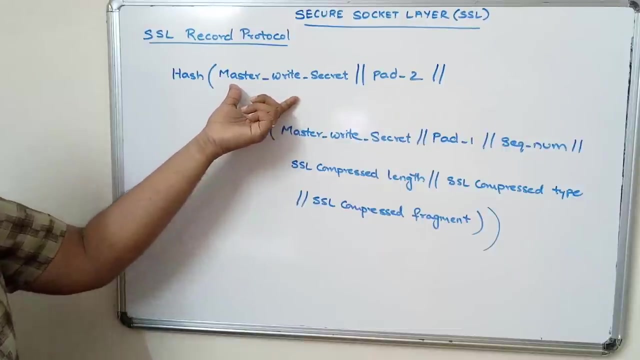 Appended with pad. 1. Expanded with pad. 2. appended with the sequence number which is appended with the compressed length, the SSL compressed length, appended with SSL compressed type, appended with SSL compressed frame. So this is the equation we are using to generate the MAC in this SSL Right. So here let us see one by one. So first one is master write secret. So here the master write secret means the shared secret key. It is a shared secret key between the client and server. 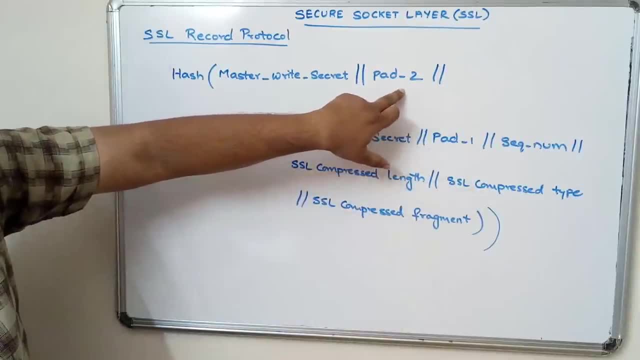 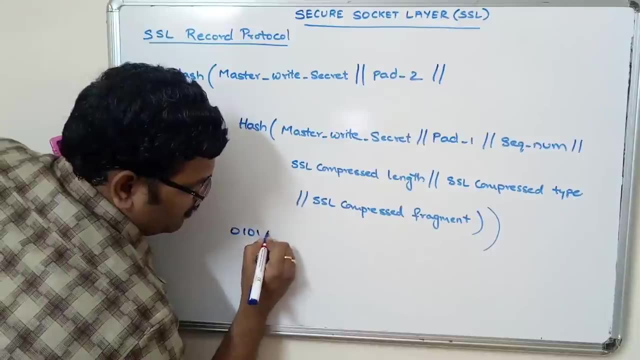 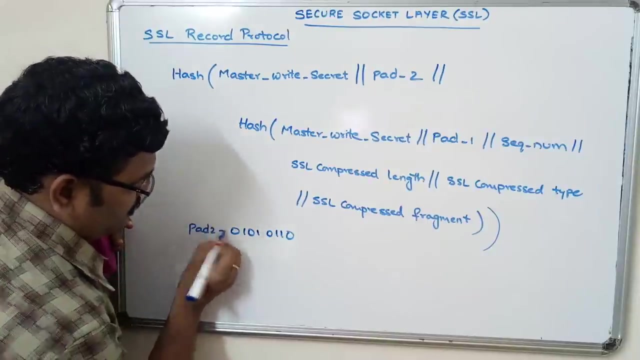 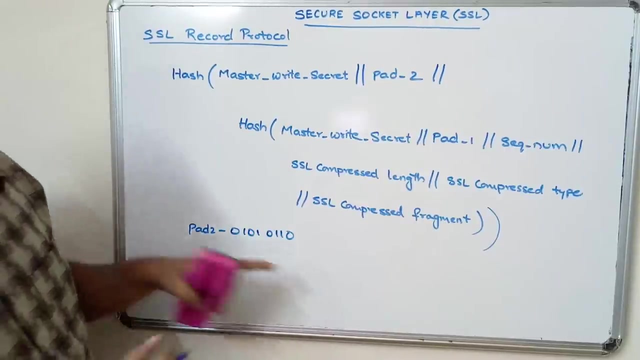 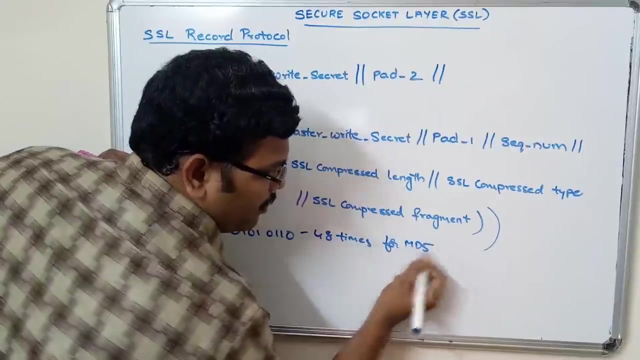 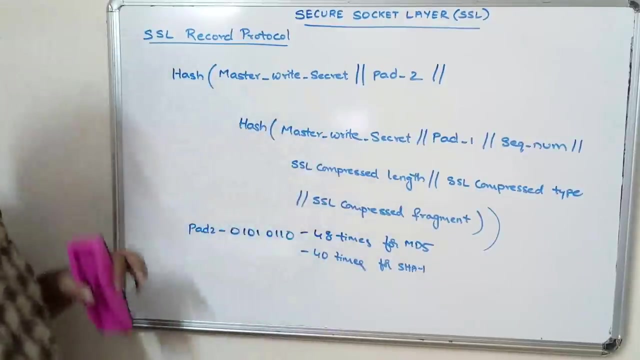 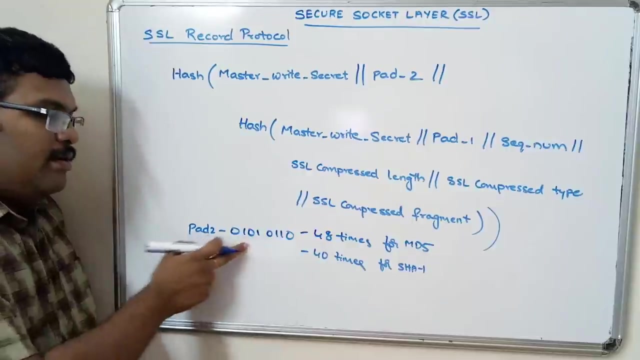 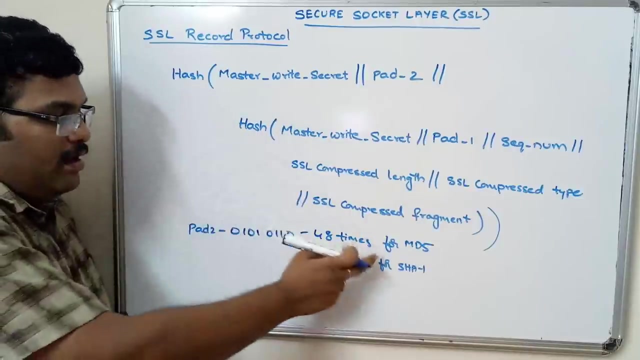 And the pad 2.. Here the pad 2 is the shared secret key. So pad 2 means pad 2 is the byte sequence repeated 48 times for MD file, 48 times for MAC. So this is the pad 2.. That means repeating this particular byte sequence 48 times for MD file algorithm. If you use the MD file algorithm to generate the MAC, we have to repeat it for 48 times. 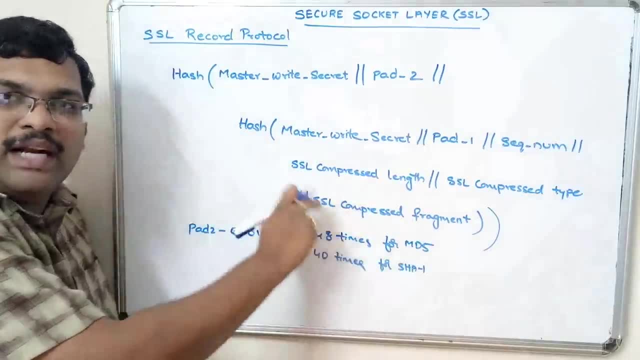 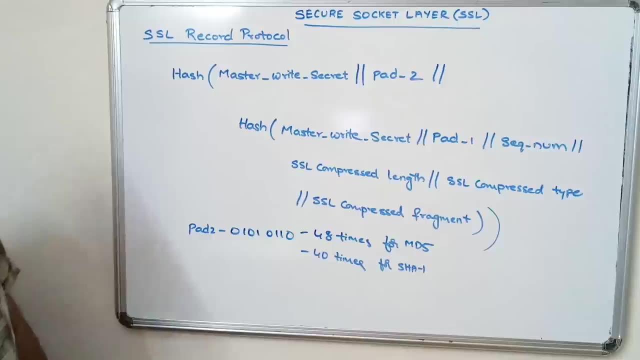 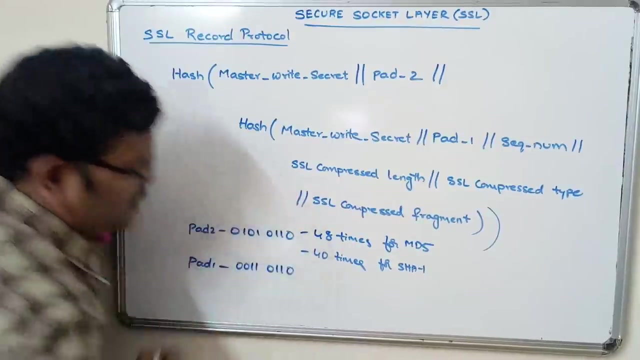 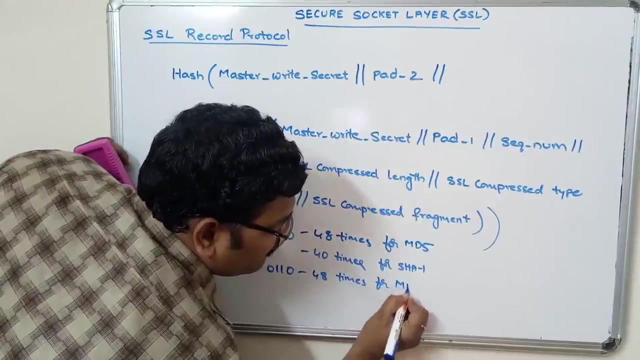 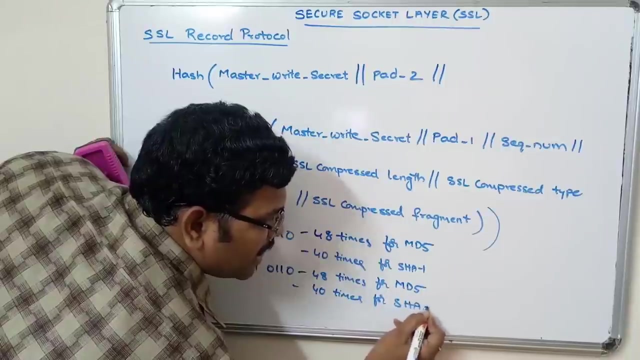 If you use SHA-1 algorithm to generate the MAC we have to use, I mean we have to repeat this byte sequence 40 times Now, pad 1.. Repeat this byte sequence: same 48 times for MD file, 40 times for SHA-1.. Right. 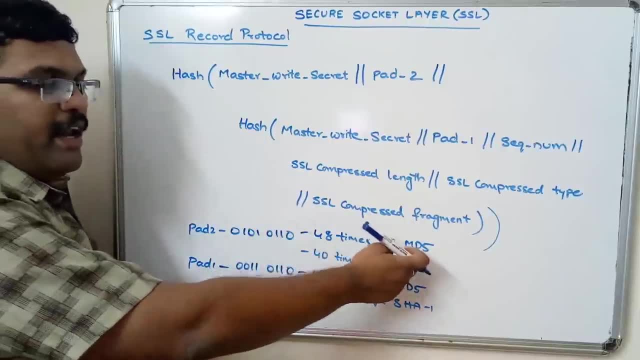 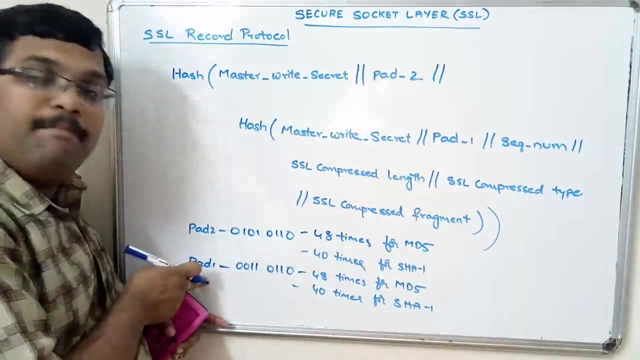 So, depending on the algorithm we are using, If we are using to generate the MAC, we have to repeat this particular byte sequence for pad 2 and pad 1.. And the master write secret. So here it is not a master write secret. 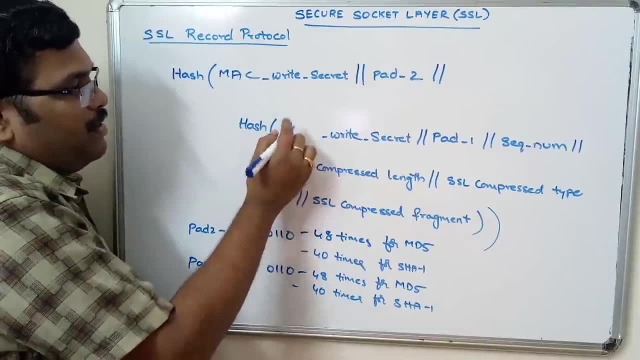 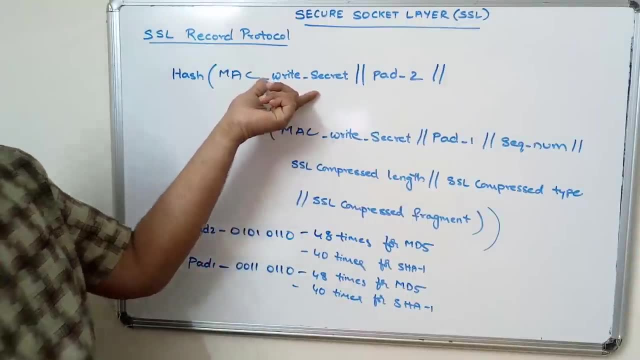 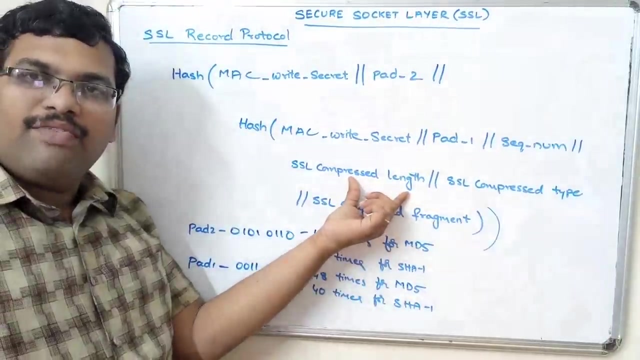 We can call it as a MAC write secret. So MAC write secret. So this is the shared key. So this is the shared key between the client and server Right. Next sequence number: we know The compressed length If the any compression algorithm. 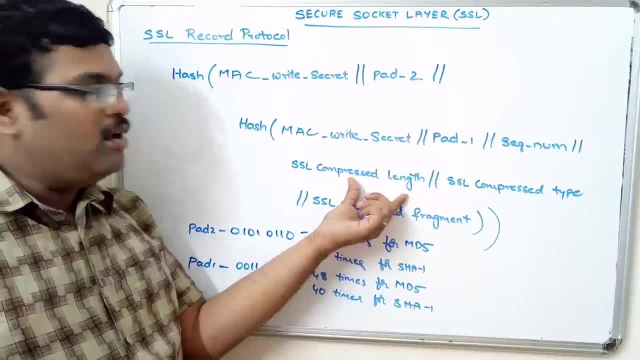 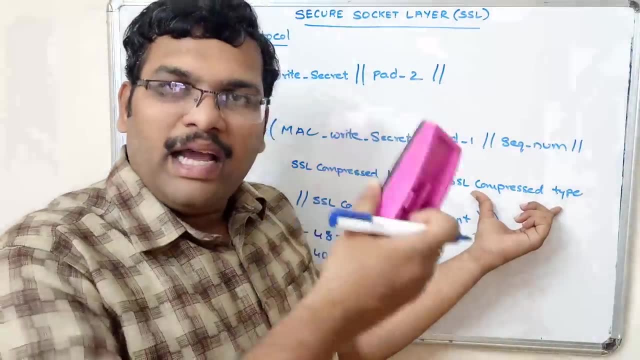 If the compression algorithm is applied, the length of the compressor fragment. if it is not applied, we can simply write it as a plain text. length of the plain text. The compressor type, that means the higher level protocols, higher layer protocols to which the fragment will be processed. 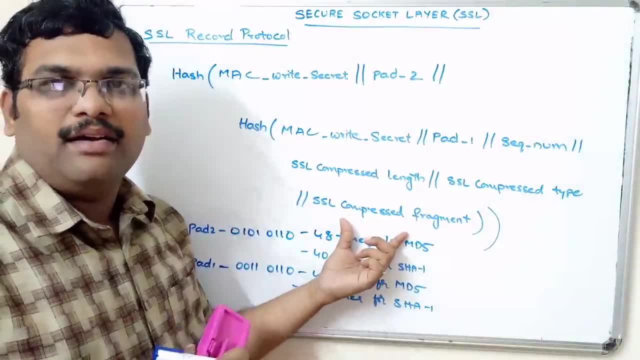 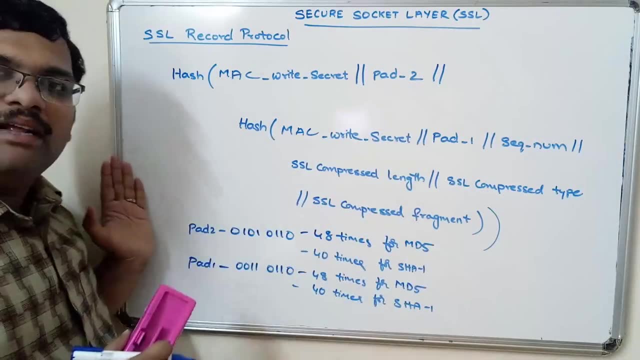 And the compressor fragment, the actual fragment, the data, the compressor data. So, applying this MAC, the hash algorithm for all these things, we will get the MAC. That MAC will be appended to the compressor, We will get the compressed length. I mean compressed data.